Hi guys. so today we'll be looking at how to solve a simultaneous equation using a method known as the Cramer's rule. So the Cramer's rule is used to solve a 3 by 3, a 2 by 2, even a 4 by 4 matrix, and I'll show you how that is done in a few. 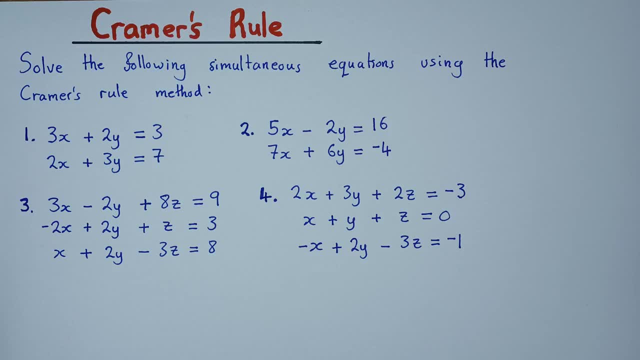 seconds. So the first thing you have to know is that you have to know how to determine the determinants of a 2 by 2 matrix, a 3 by 3 matrix, depending on which type of matrix you are looking at. So it's very important that you know how to. 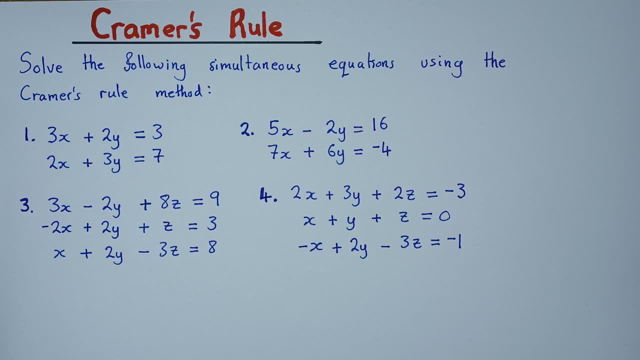 find a determinant. hence I've dropped a link in the description, just in case you don't know how to find the determinants. So go through that first, then you can come here and go through how to find the values of certain variables given simultaneous equations. Ok, So we 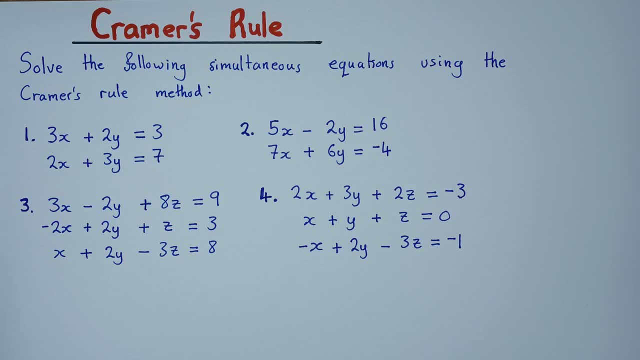 have some examples. The first two examples are representing a 2 by 2, two variables, and the second one is the second. two examples are representing a two by two and the second one is the second. two examples are representing three by three, three variables. So let's start with the two by twos. 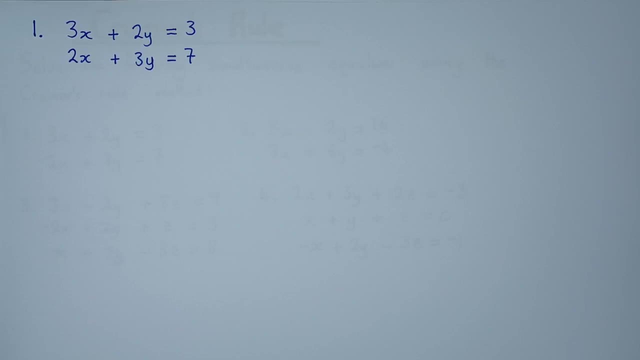 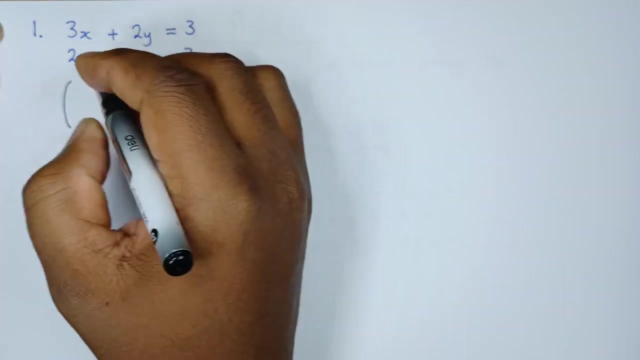 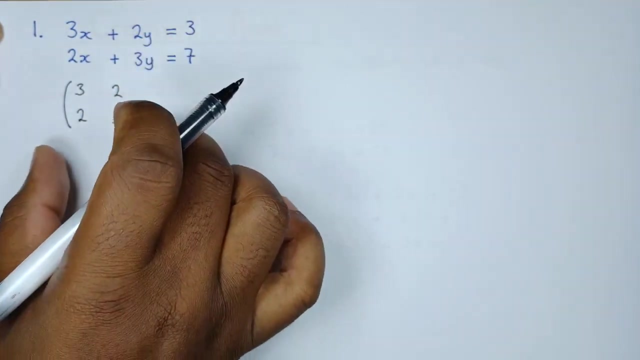 Okay, so here's our first example. So what we're going to do is we're going to form a matrix. This matrix will, of course, be the first. one will be a two by two, which will be: we'll have three there, two there, we have two there three. Now, these matrices, this matrix that. 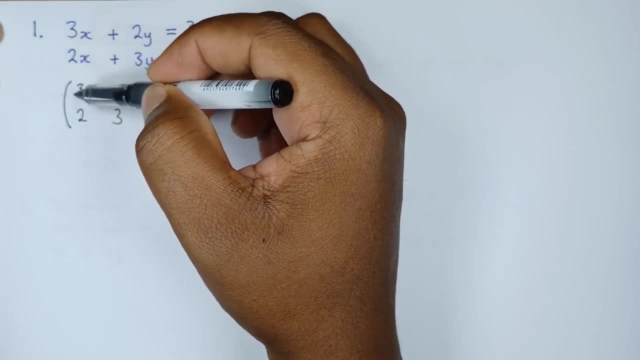 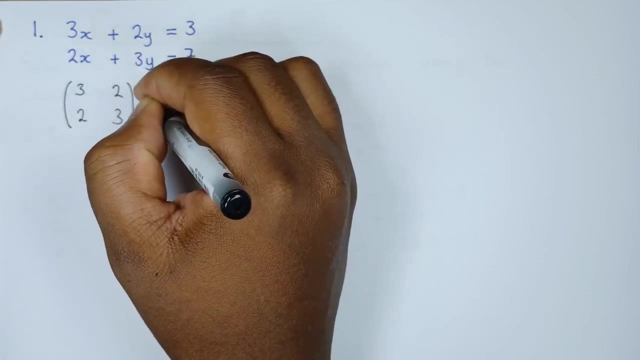 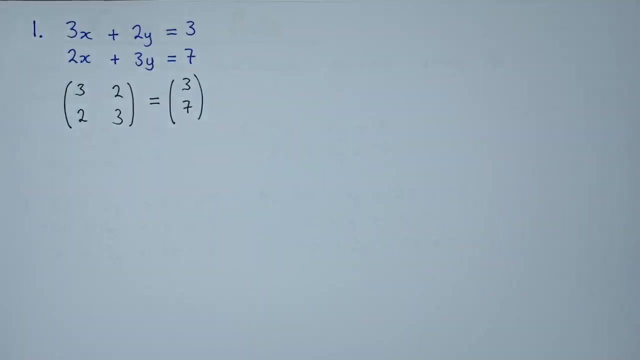 I've formed, rather, is just formed by the coefficients: the three, the two, which is that one, the two, the three, which is that one, like that. Then I'm going to do this. this whole thing is equal to whatever we have here, which is a three and seven. okay, 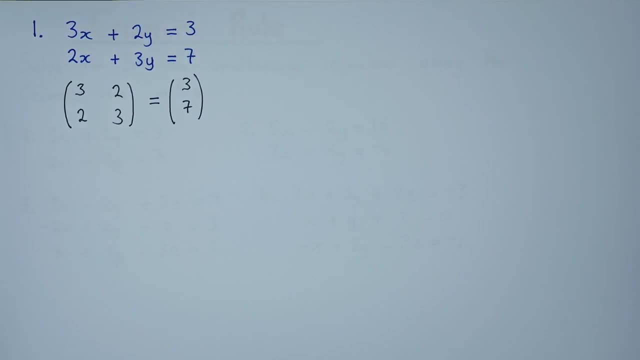 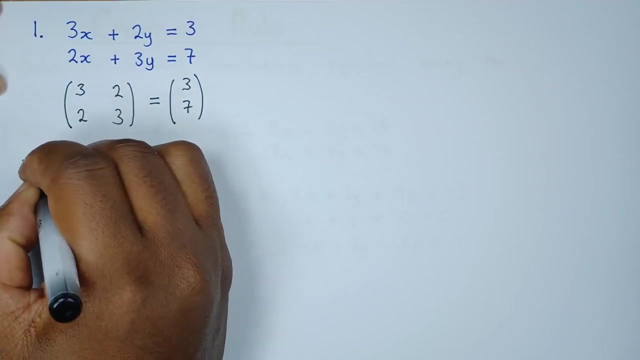 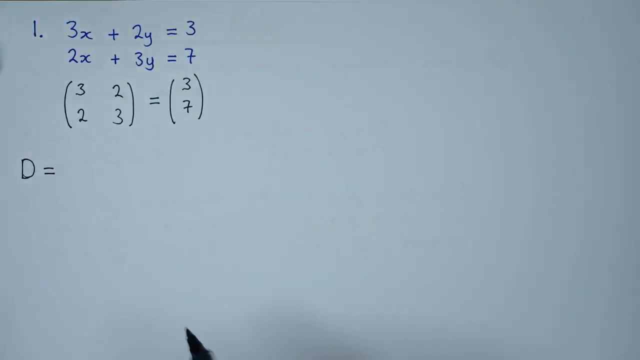 So the first thing we're going to do is we're going to find the determinant of this matrix. Now, the determinant of this matrix, I'm going to call it d So d will be given by the product of the measure, that minus the product of the minor diagonal. Hence the determinant will be nine minus four, That is. 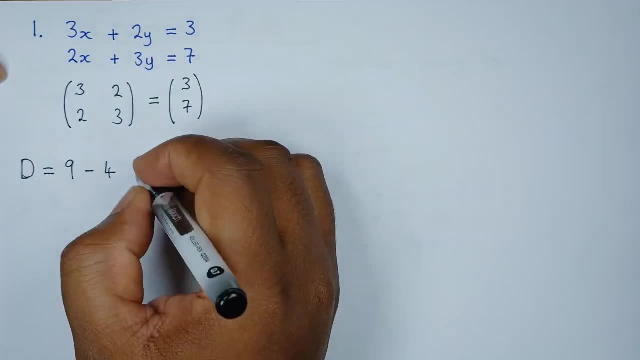 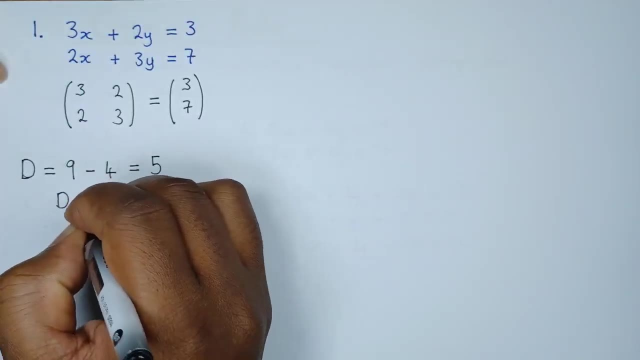 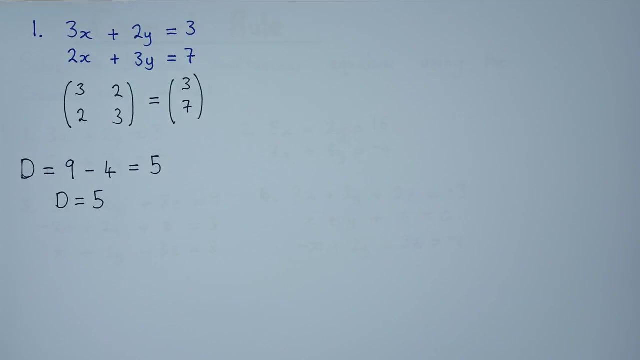 this times that which is nine, that times that which is four, we subtract the two. Hence our determinant in this case is five. So we have found the value of d to be five. Okay, let's look at what else we need. So the next thing we're going to do is we're going to create the next matrix. 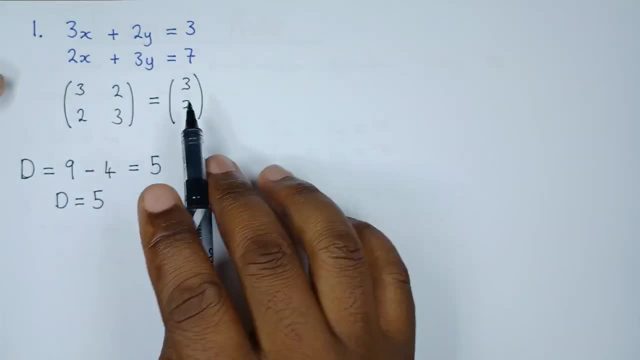 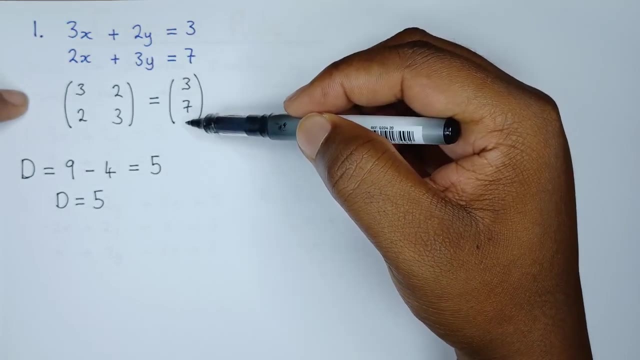 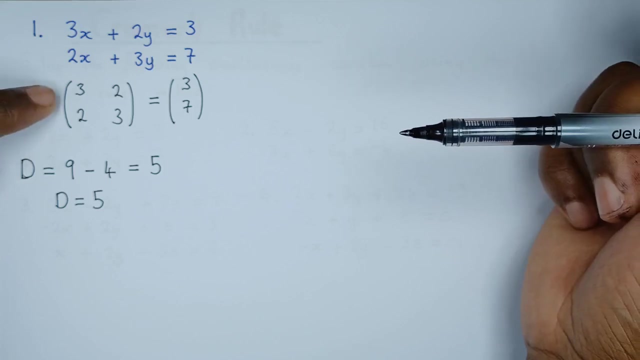 Now, the next matrix we're going to create will look like this: These values that you see here, this matrix, the two by one matrix, which has a three and a seven, Since we want to find the value of x, the value of x, the determinant of the value of x will be dx. So what you're going to do is: 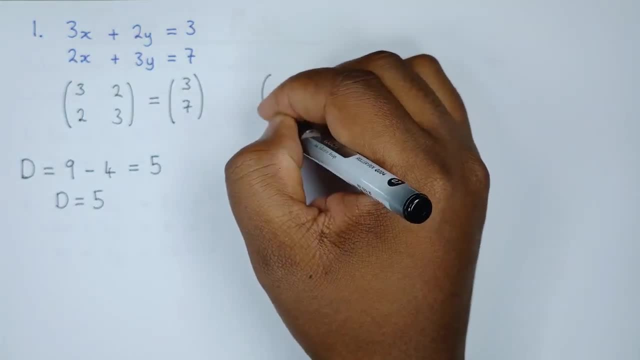 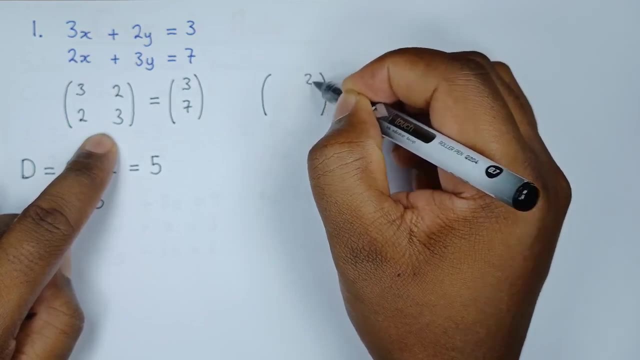 you're going to create another matrix which will look like this. From this matrix, the two by two that we have here repeat the values of y As they are, but for the values of x, instead of writing the three and the two, since we're 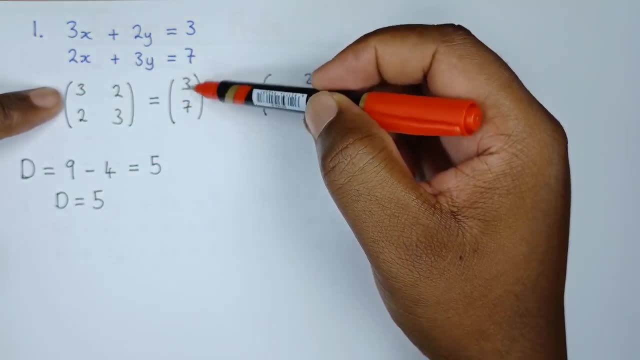 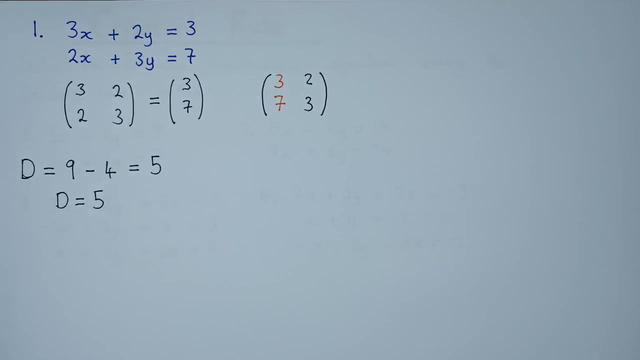 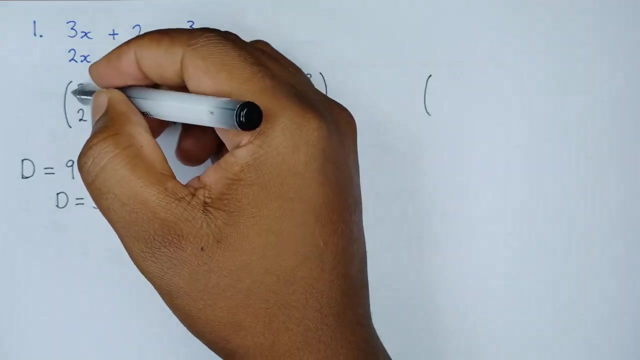 finding the determinant for the x values. what you're going to replace it with is these two values that you have here, which is a three and a seven. Now, this will also work in the same way when we want to find the value for dy. So you'll have the values. of x will be maintained, which is 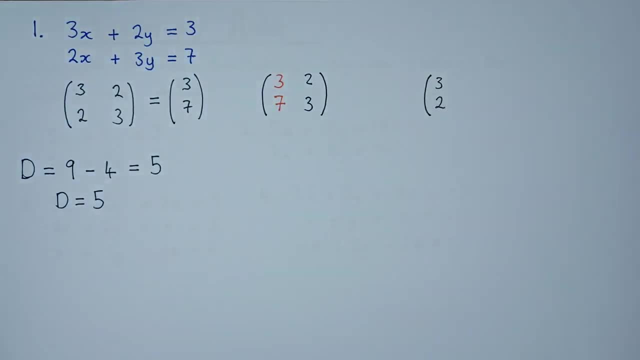 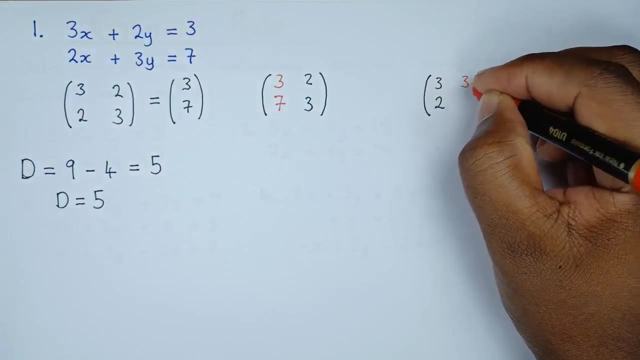 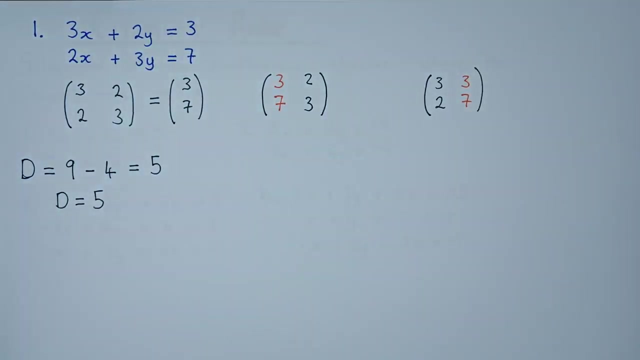 three and the two, but it's the values of y- will equal the equation of d and w. So how would this the coefficients of y, which will be replaced by this, which is a three and a seven, like that. so i hope it's making sense. so, applying that concept. the next thing now, what we're going to do. 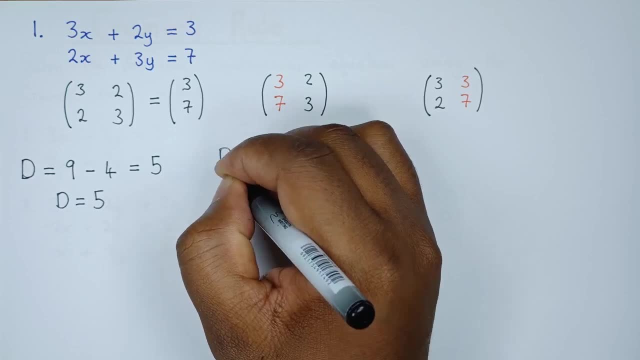 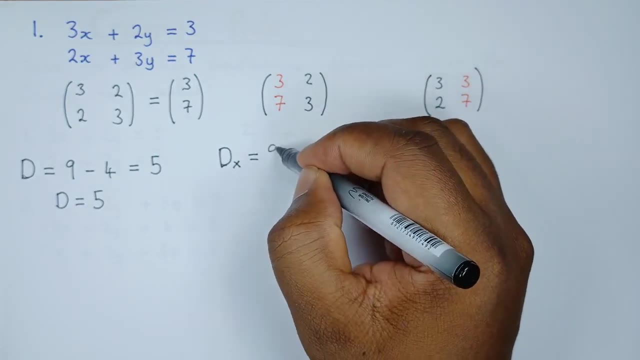 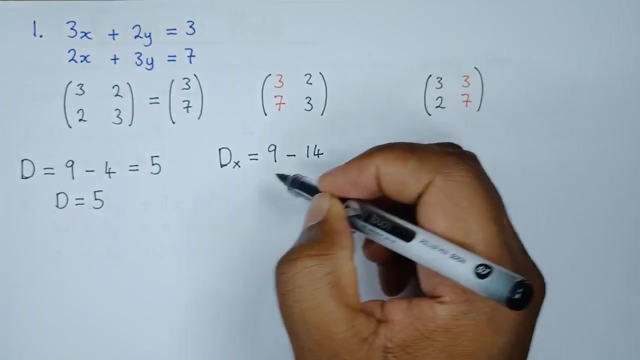 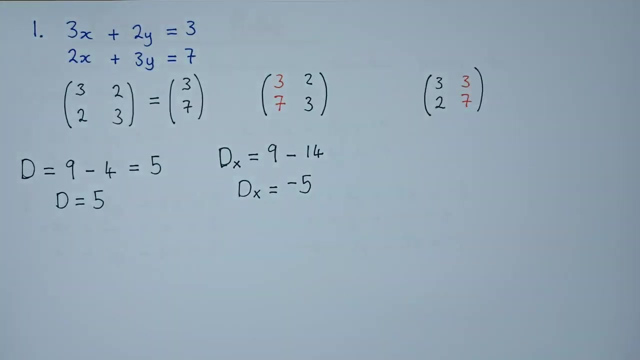 is, we're going to find the determinant. so this determinant is dx. so the term dx will be found by three times three, which is a nine minus seven times two, which is 14.. so dx will be equals to negative five. like that, we're going to move on to this, this one, here as well, applying the same thing. 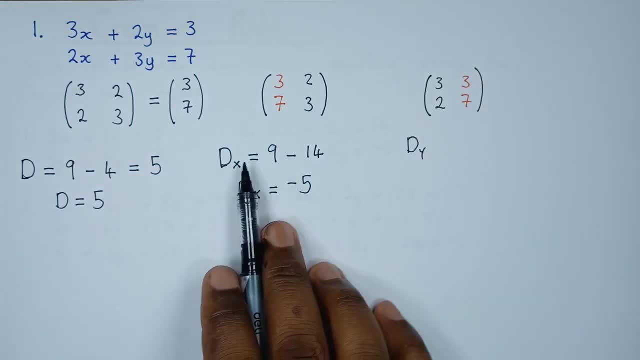 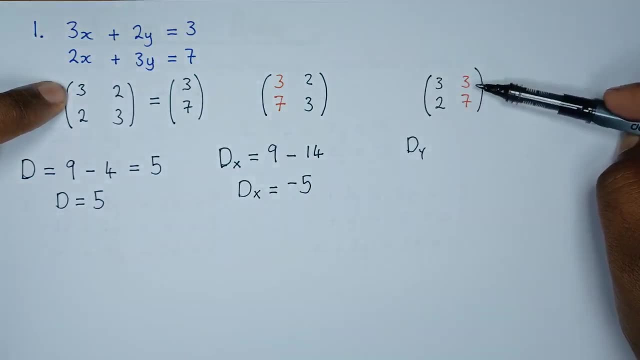 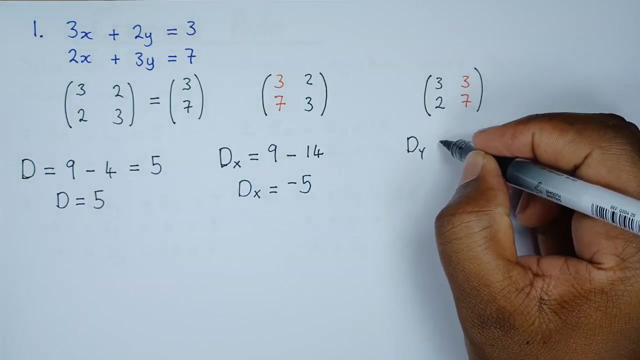 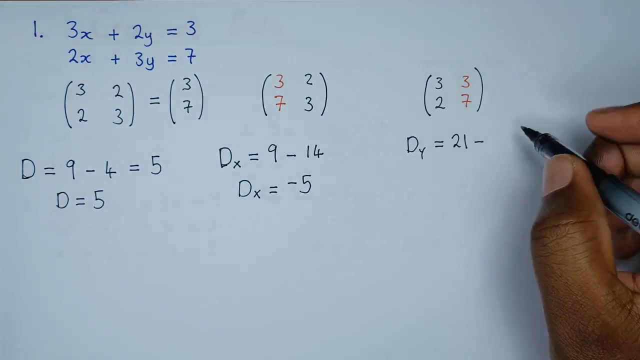 so this is d, y. so this one is dx, because we substituted the coefficients of x with whatever we have on this side. this one is dy because we substituted the values of the coefficients of y with whatever we have on this side of the matrices that we formed there. so dy will be equals to 3 times 7, which is 21, minus 2 times 3, which is 6, hence dy. 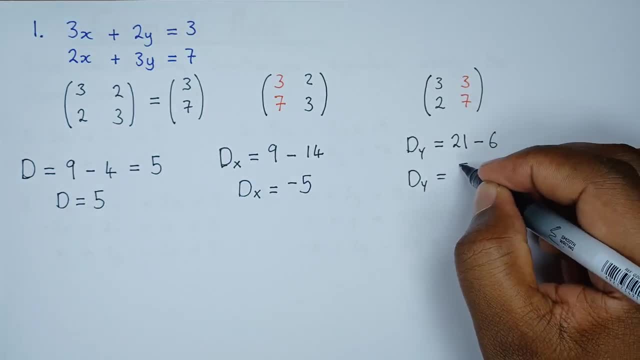 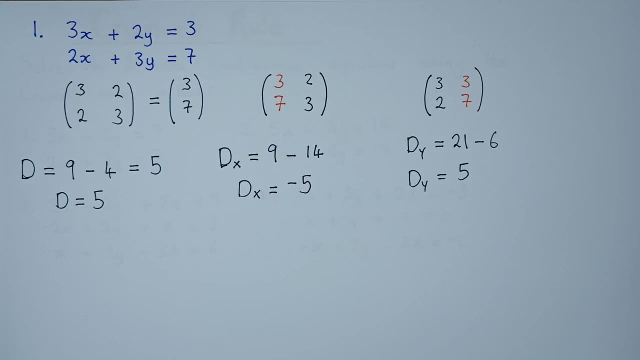 is equals to 5, like that. so now that we have the three determinants, let's see how we can find the values of x and y. so finding the values of x and y, this is the easy part. the difficult part is finding the determinants. so to find the value of x. 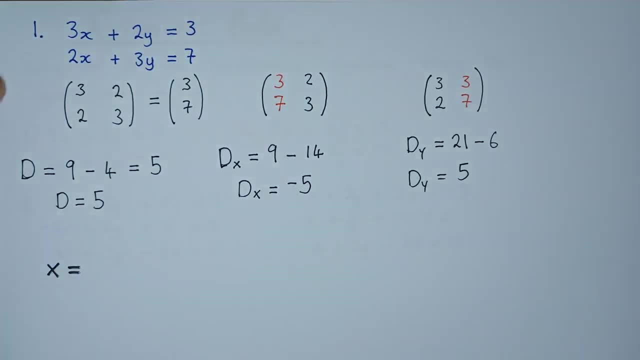 the value of x will simply be given by dx over d, just d. so to find the value of x, our dx, we found negative 5 and our d, remember our d was 5. so subtracting the two, the value of x is negative 1. to find the value of y, we're going to say 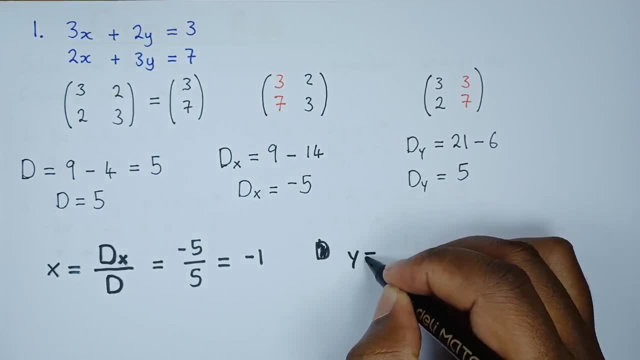 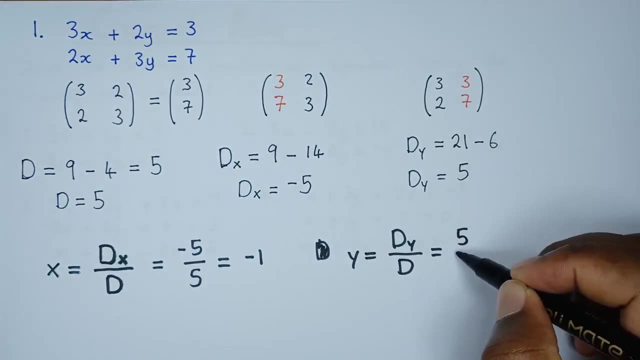 oh, sorry, sorry. y is equals to dy over d. now our dy in this case is just 5 and our d is also 5, like that. so meaning that the value of y is 1. so that's our solution. set x is equals to 1. 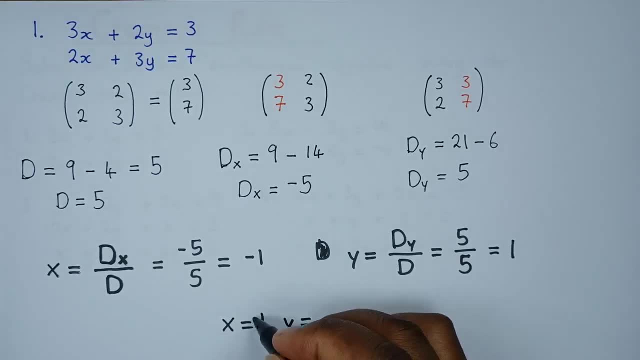 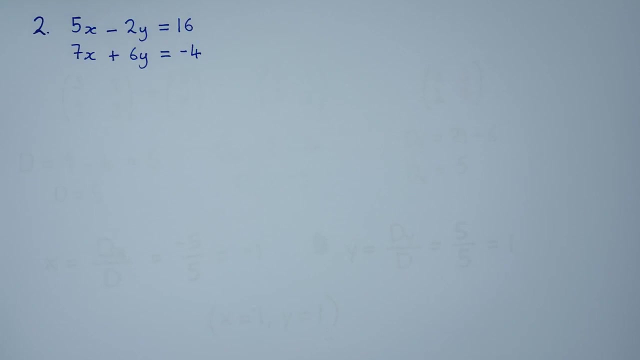 and y is equals to, so x is negative 1 and y is equals to 1, just like that. so let's do the next example as well. so for this example, i would urge you to pause the video, try it out, just like we did in the previous example. then see if you get whatever i'm going to find as well. 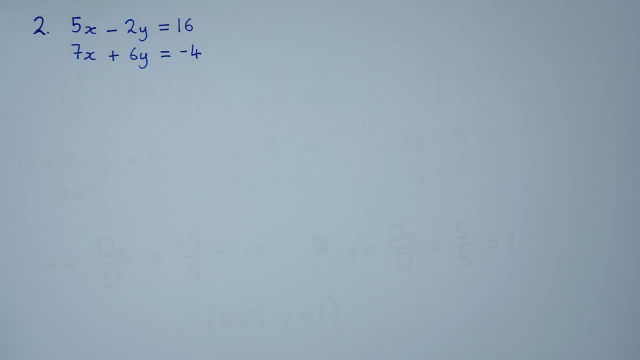 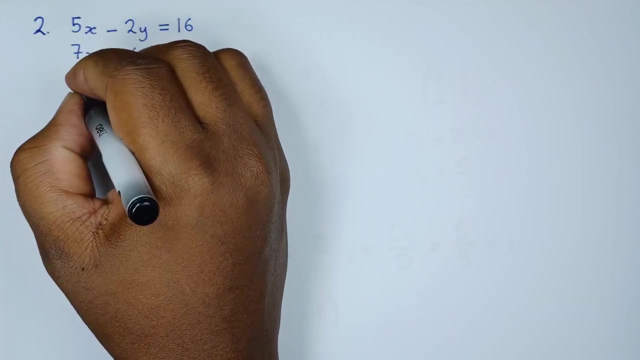 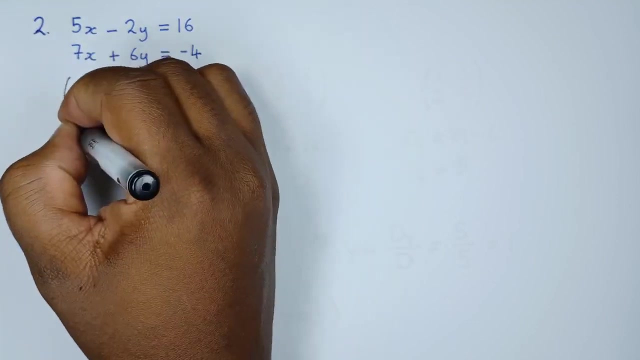 okay, so assuming that you just did that, so let's go ahead and solve it now. so we form the matrix. the matrix form in this case will be 5, 7, negative 2 and 6, and on this side we'll have the matrix 6 negative 4. 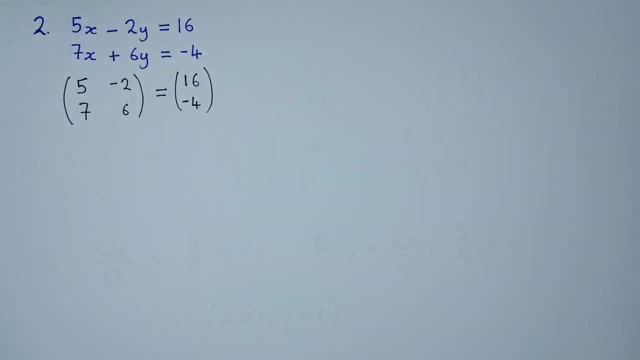 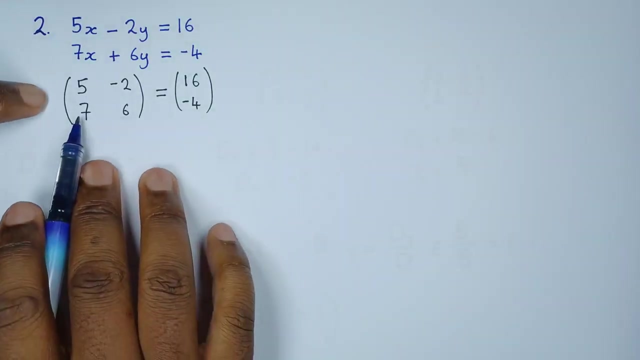 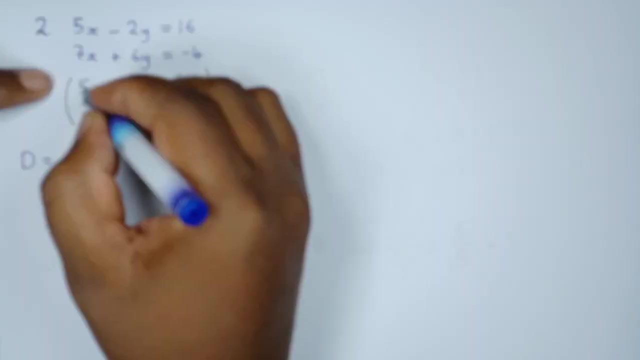 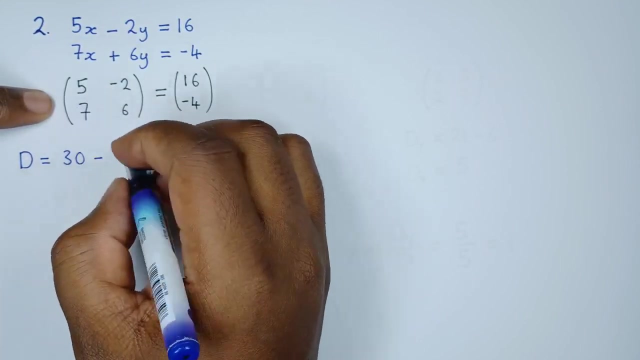 so the first thing we're going to find is d. now, remember, d is found by the determinant of this matrix that we have here. so d will be equals to 5 times 6, which is 30 minus 2 times a negative. 2 times 7 should give us negative 14. 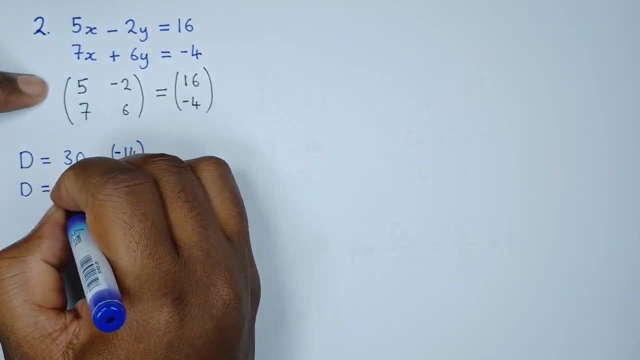 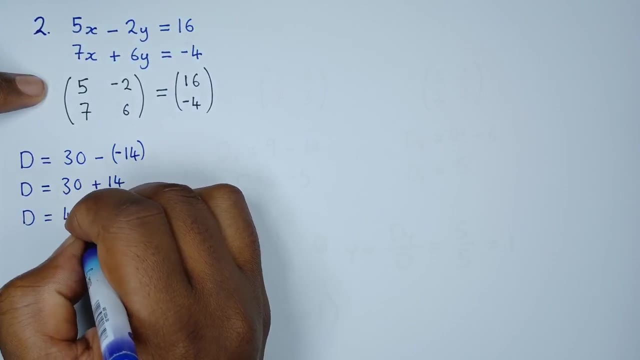 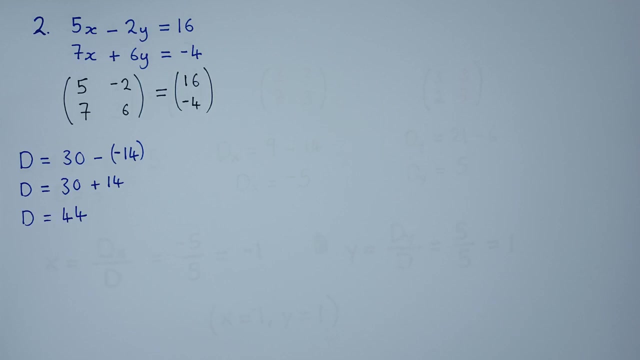 so the value of d will be 30 plus 14. hence d is equals to 44, like that. so we found the value of d. let's find the value of d, x. so we're going to rewrite the matrix, so the matrix will be for the values of x. 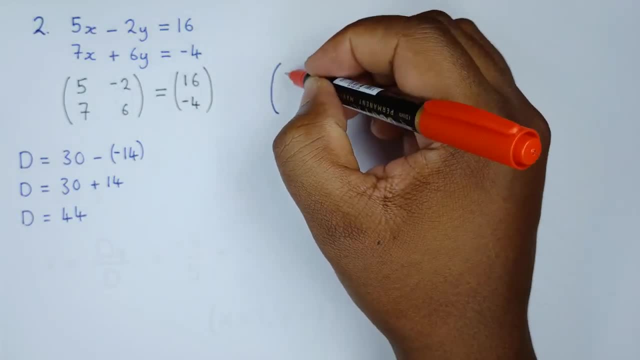 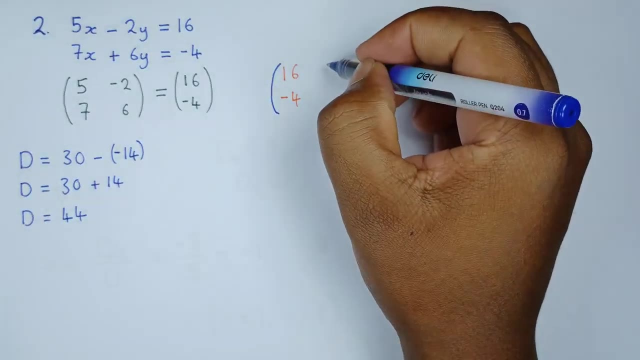 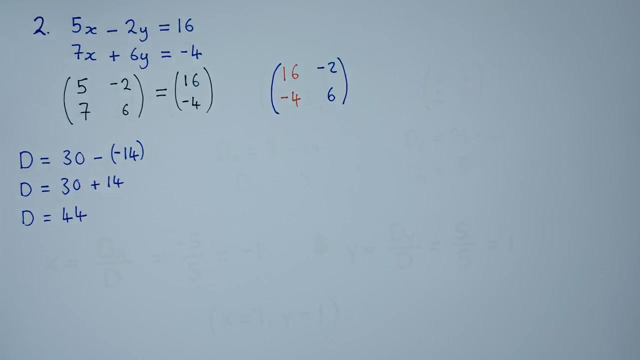 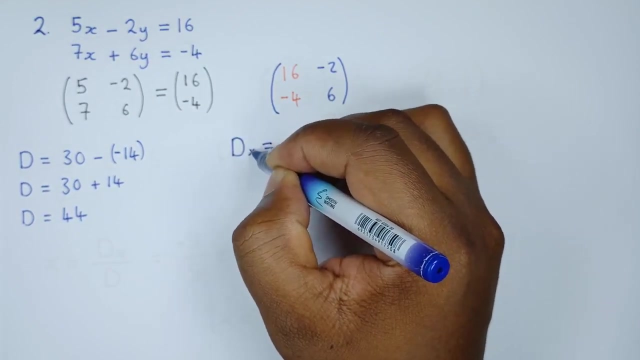 we shall replace them with these values that we have here, which is 16 and negative 4, like that. then we write the values of y as they are, which is negative 2 and 6. so this will give us dx. dx will be equals to. so let's find the determinant of dx. 16 times 6 should give us 96. 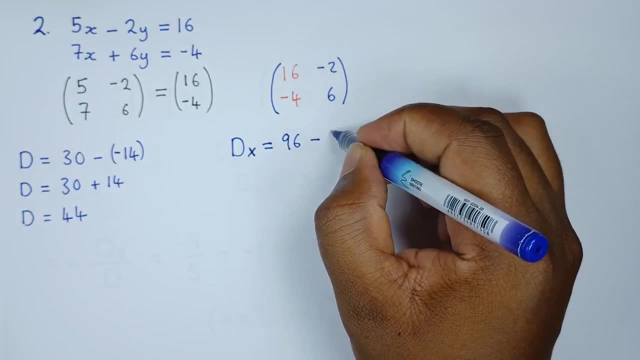 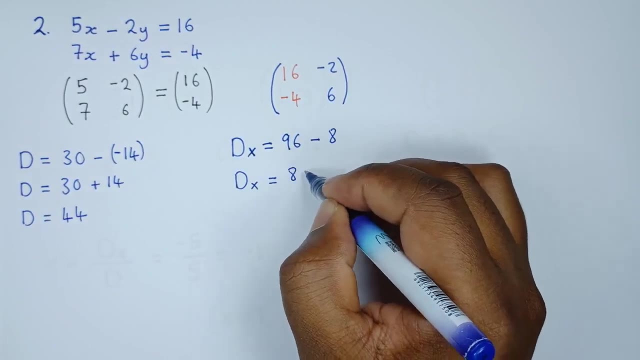 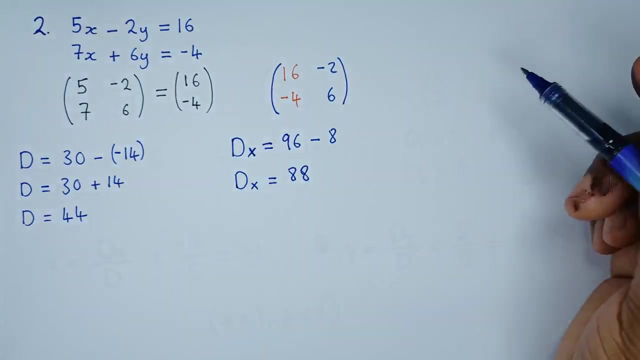 minus negative, 4 times negative, 2 is positive, 8 like that. so the value of dx will be equals to 88. so the value of dx is simply 88. let's form the next matrix for dy. so for dy we maintain the coefficients over x, which is 5 and 7, but for the coefficients of y 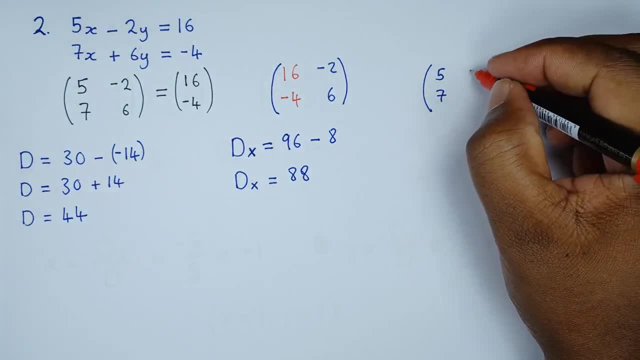 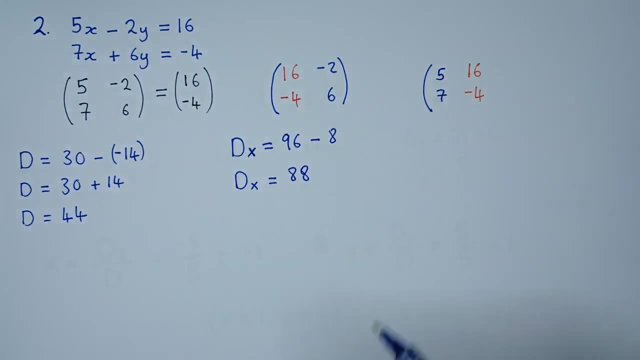 we shall replace them with 16 and negative 4. so here we have 16 and negative 4. like that, then dy will be equals to. so if we multiply 5 and 4, so 5 times 4 will be, is negative 20 minus. if we multiply 16 and 7, we seem to get 112, so that 112. 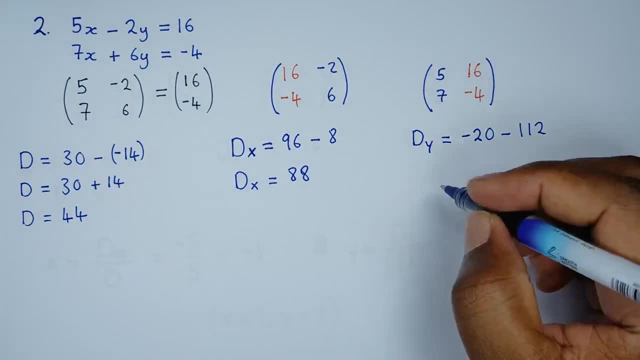 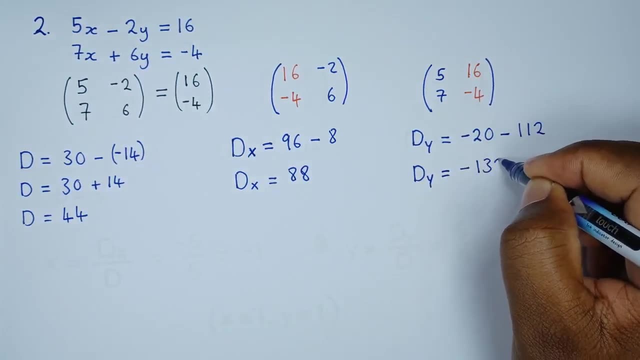 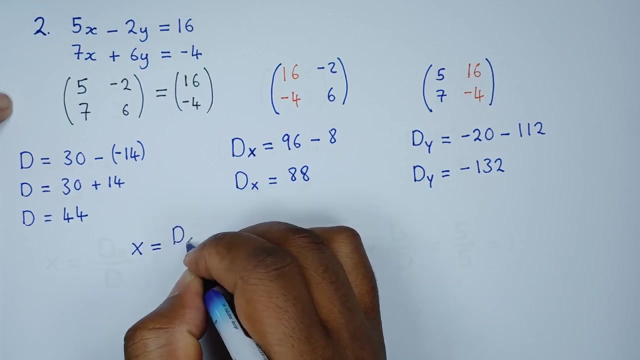 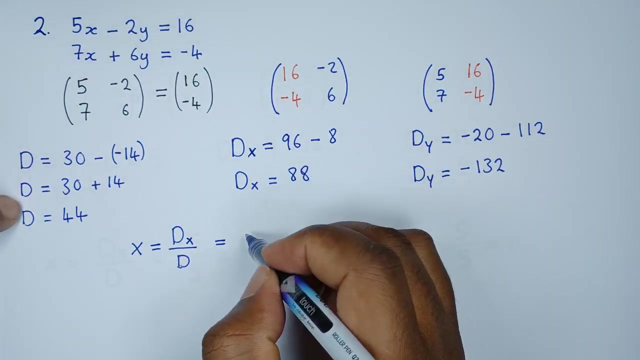 negative 20 minus 112 should give us dy being equals to negative 132, like that. so this is the easy part, or rather, this is the difficult part. the easy part is just finding the values of x and y. so x is equals to dx over d. so on the x, remember our dx is a 88, our g is 44, so the value: 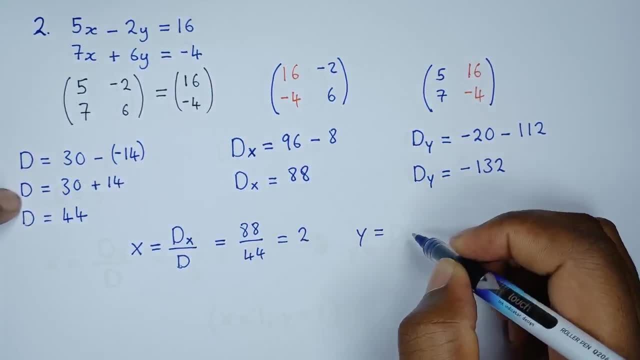 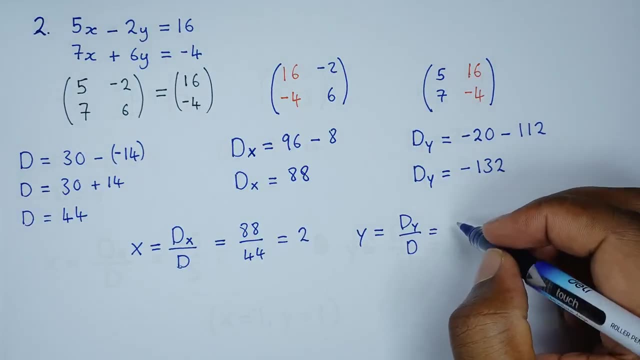 of x is simply 2. the value of y will be given by dy over d. the value of dy is simply this one here, which is negative: 1, 3, 2 and the value of d is 44. if we subtract the 2, or divide rather, we get negative 3. so that's our. 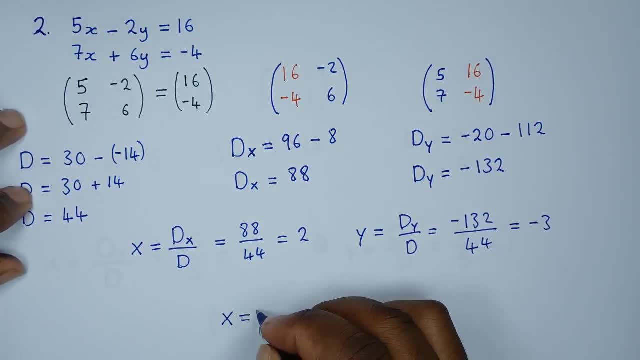 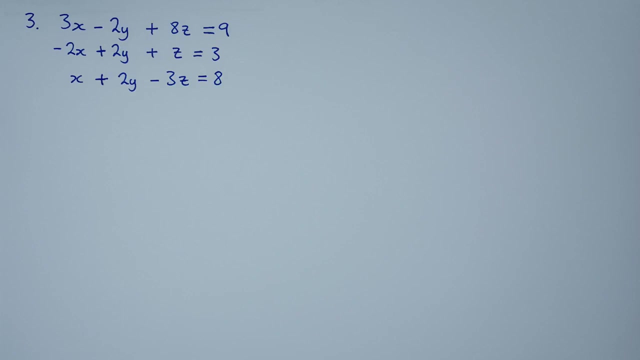 solution set the value of x is simply 2, while the value of y is negative 3. okay, so now let's quickly look at how to find determinants of a 3 by 3 matrix using the same approach. okay, so, finding the determinants of a 3 by 3 is a bit lengthy, but i'm sure you can do it, so let's go ahead. 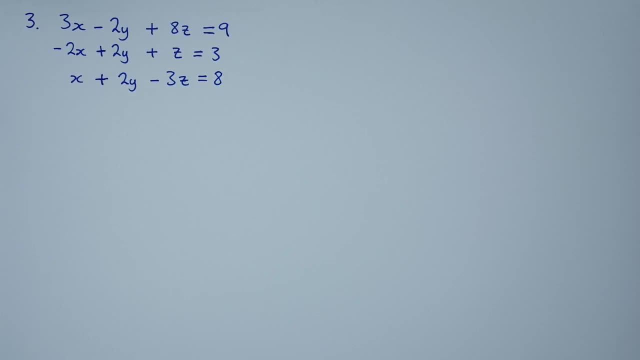 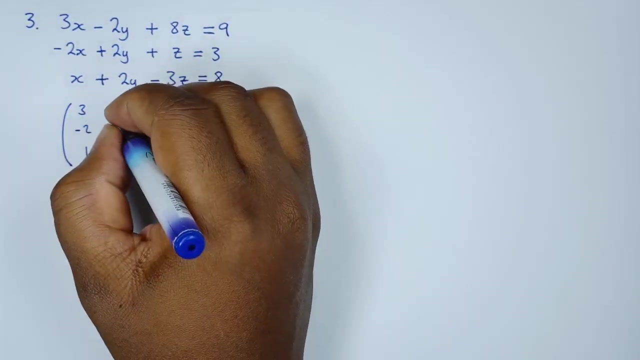 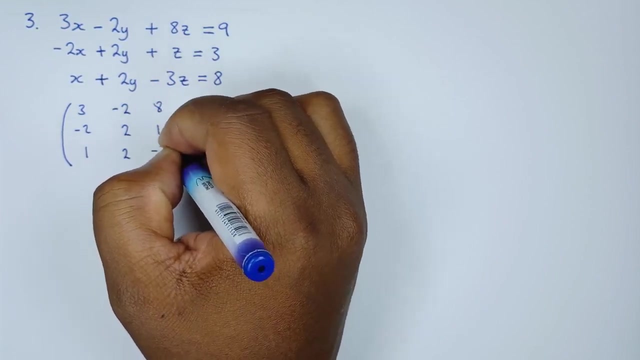 so let's create the 3 by 3 matrix. so the 3 by 3 matrix will look like this: we have 3 negative 2, 1 negative 2. we have a 2 there and a 2 here. we have 8: 1 and negative 3. 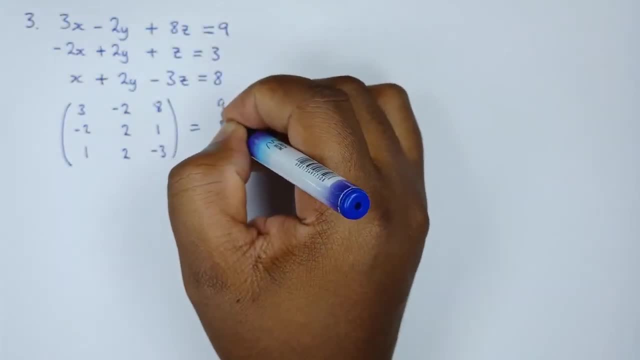 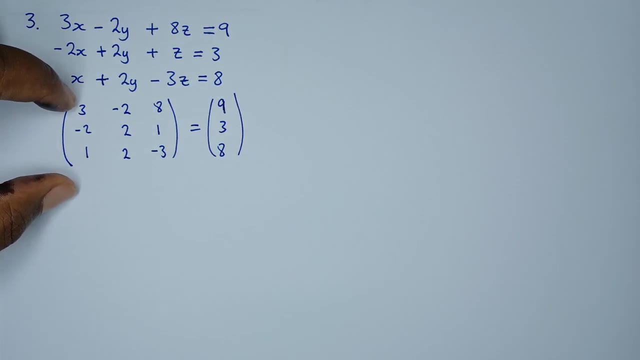 what we have this side is simply 9, 3 and 8. okay, so we're going to find the determinant of this matrix, and that determinant that we'll be finding will be known as our d, of course. so let me form the 3 matrices that we are supposed to find that. 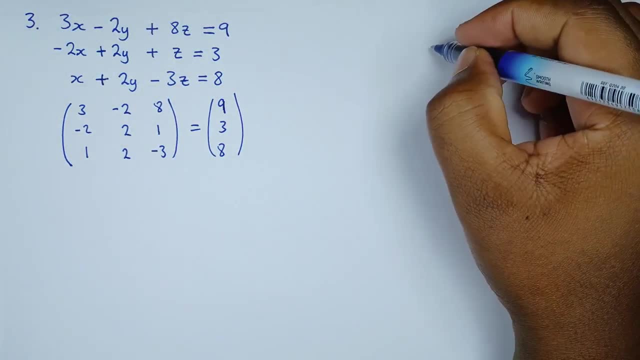 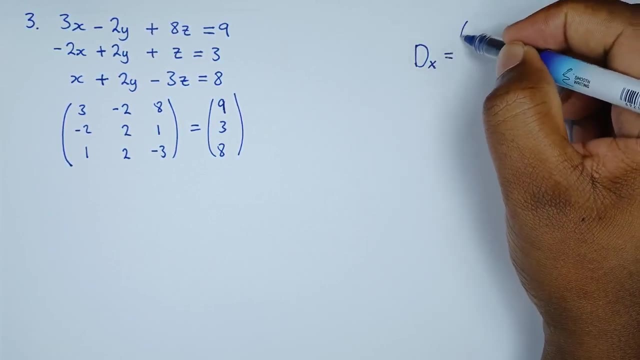 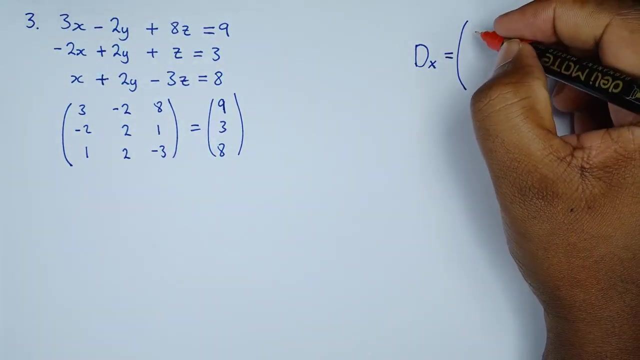 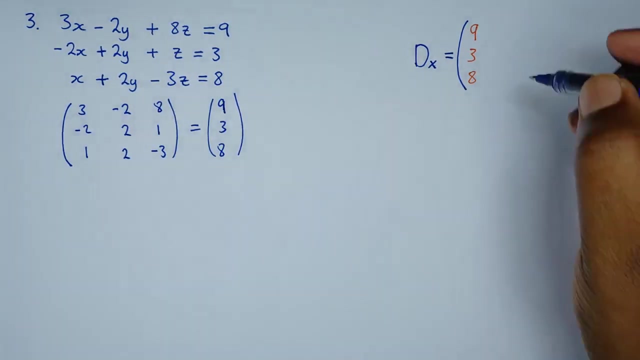 will guide us into our process. so the first thing we're going to look at will be dx. now, remember dx. this is when we have to replace the coefficients of x with these values that we have here. so that's, the coefficient of x in this case will become 9, 3 and 8, then everything else as it is, so we have a. 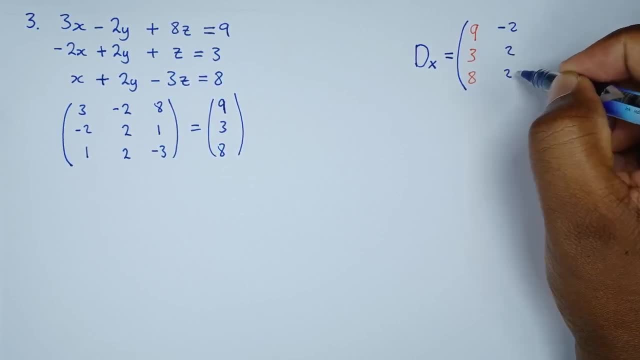 negative 2 there. here we have a 2, here we have a 2 again. so 8: 1 negative 3. okay, the next thing we're going to look at is dy. so dy, the matrix form will be: we maintain the coefficients for x, which is 3. 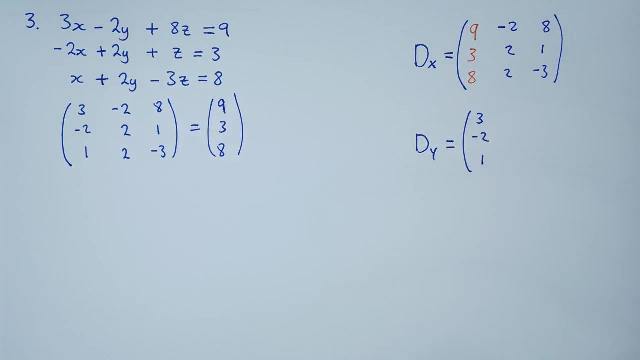 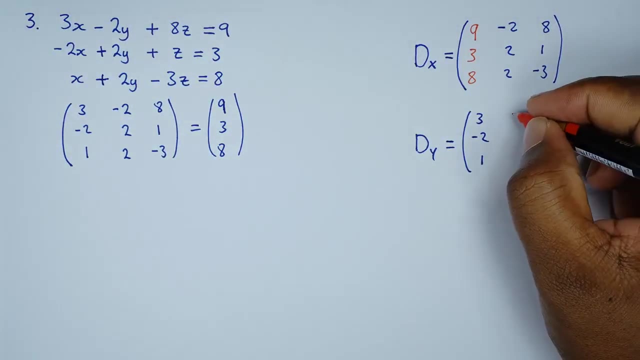 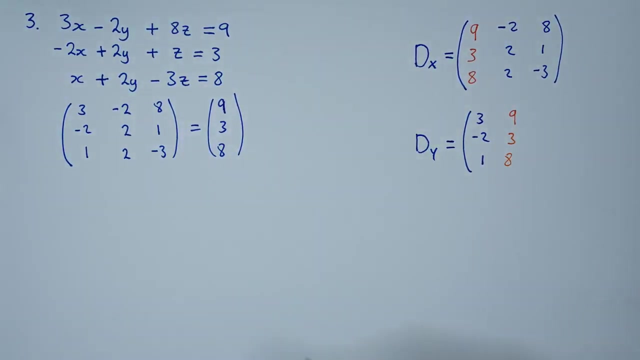 negative 2: 1 for y. the coefficients for y, which are these ones that we have here. we're going to substitute them with this, which is a 9, 3 and 8 like that. the next thing we're going to look at is, of course, the coefficients for z, which we just maintain as they are, so 8, 1 negative 3. 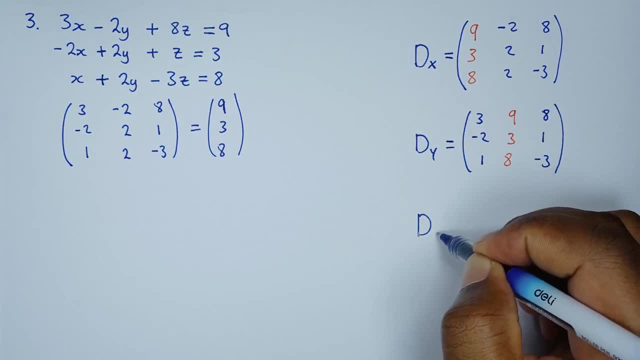 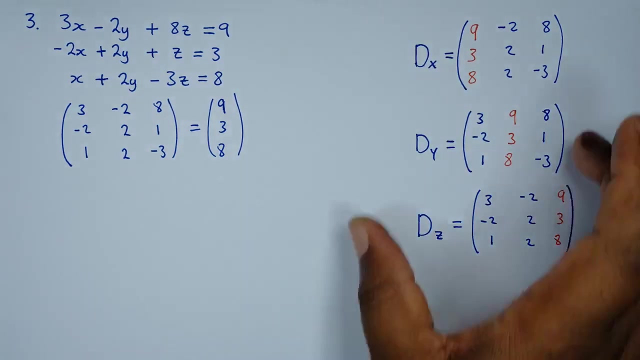 and lastly the matrix dz. so the matrix dz is going to be the matrix of x and y. so we're going to substitute the coefficients for z with 9, 3 and 8, like that. so the determinants that will come from these three matrices, this is what we get as our dx, dy and our dz. but before all this, remember we: 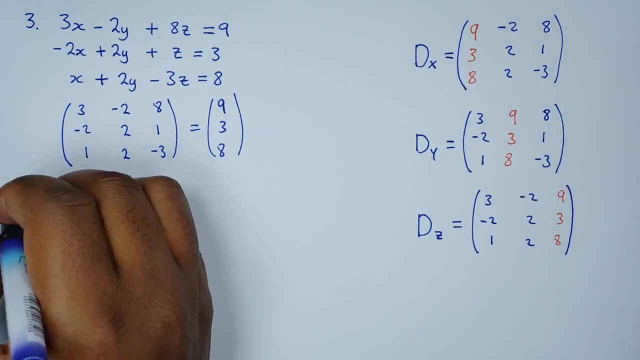 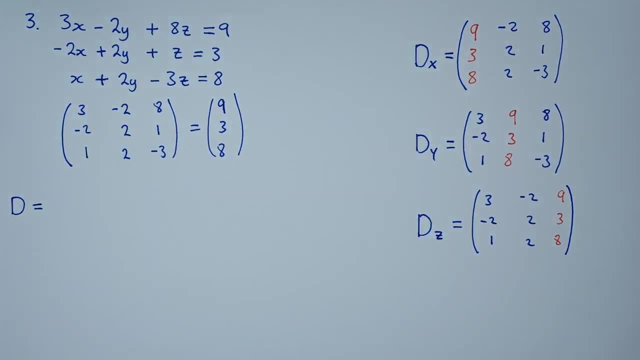 first have to find the value of d. so let's find the determinant d. so to find the determinant d, like i said, you need to know how to find the determinant of 3 by 3, so we can set this to be our positive. this is our negative, what is our positive? like that, then we get. 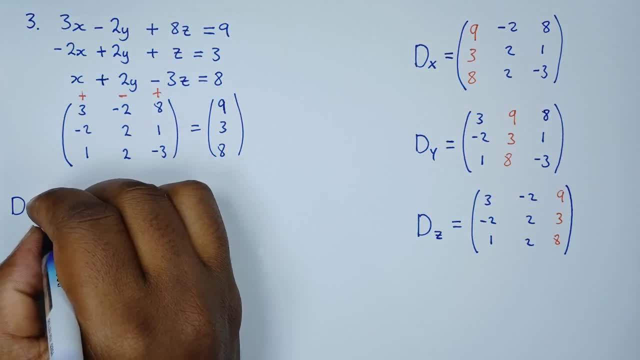 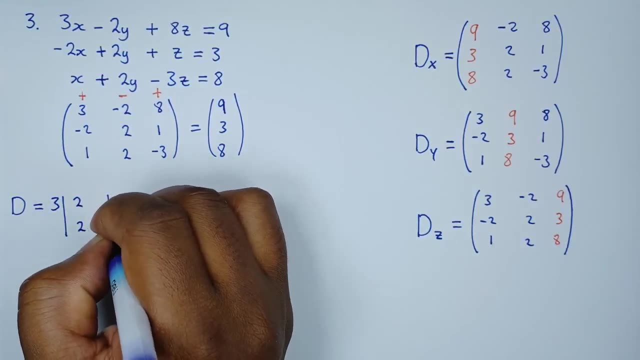 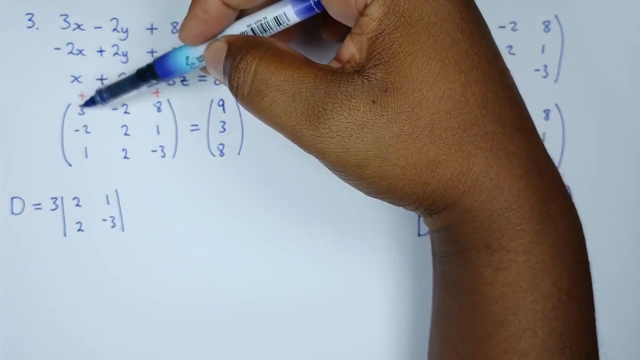 the coefficients in the first row. so the first one is a 3. we create a 2 by 2, which will be 2, 2, 1 negative 3, like that. so where are these values coming from? if we're getting these three that you see here, then we're actually forming a 2 by 2 matrix, which 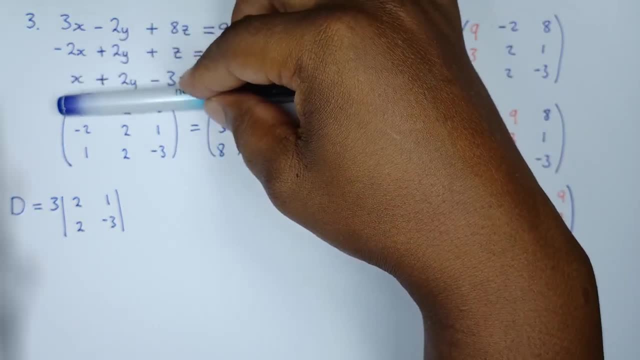 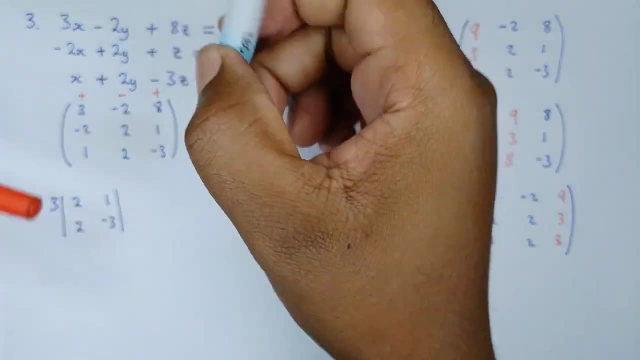 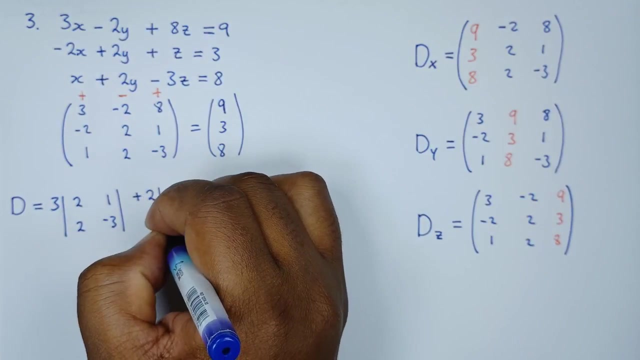 is formed by everything except that value and everything except that row and this column. so this 2 by 2 matrix which has remained here is now that we're right here. the next one is 2. remember this two has a negative, so it becomes a positive 2. so what will be the two by two formed? 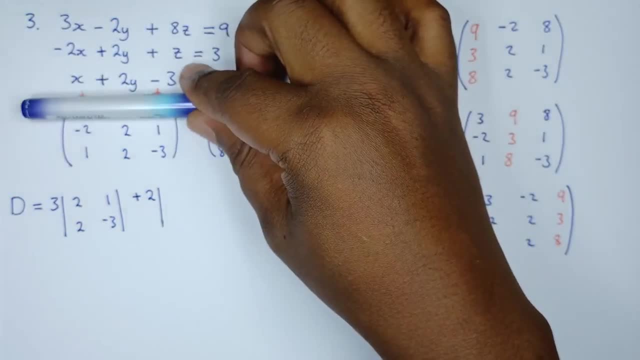 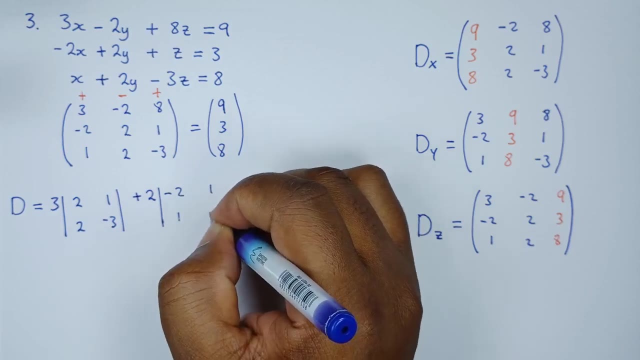 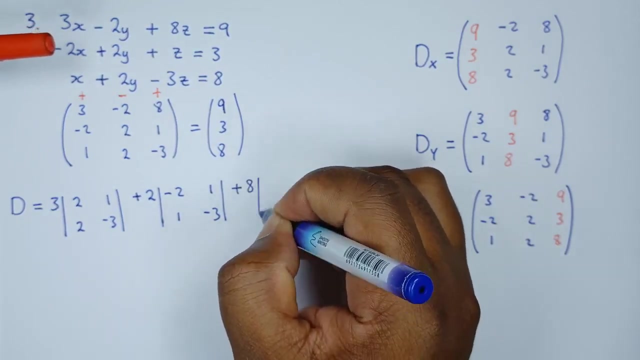 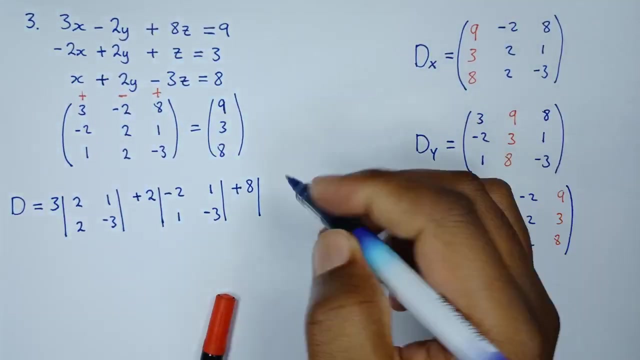 1, miss велicol, 4%. all Innen 16. 2.Christoph column. so the remaining values will be negative 2, 1, 1 and negative 3, like that. then, lastly, plus 8, the 2 by 2 formed is everything except this and this, so the 2 by 2. 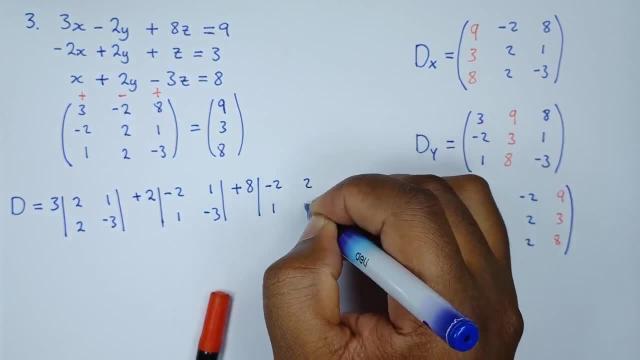 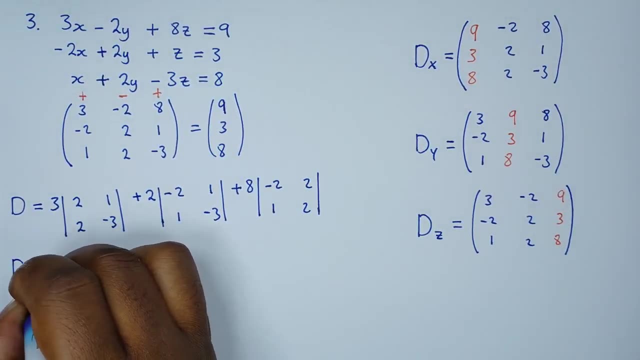 formed will be negative: 2, 2, 1 and 2. okay, from there now let's find the determinants of these 2 by 2 matrices that were formed. so we have the 3 here 2 times negative. 3 is negative 6. 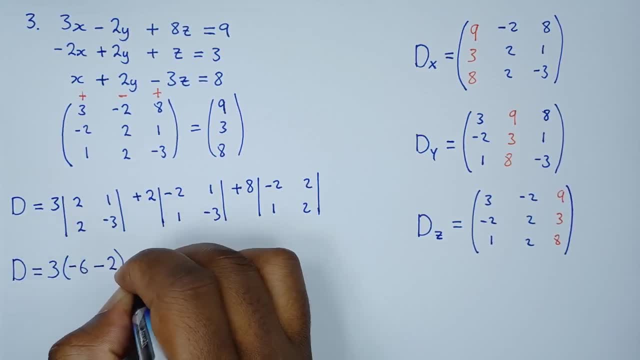 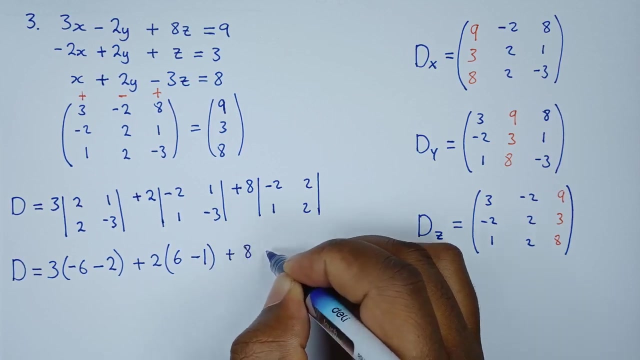 2 times 1 is 2 plus 2. negative. 2 times negative 3 is simply positive 6, 3, 3, 3. Then 1 times 1 is 1, plus 8.. So negative 2 times 2 is negative 4.. 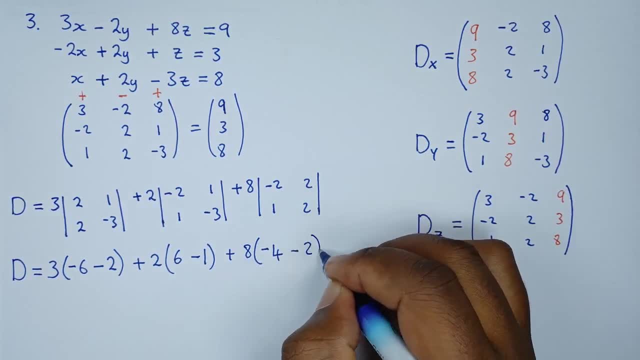 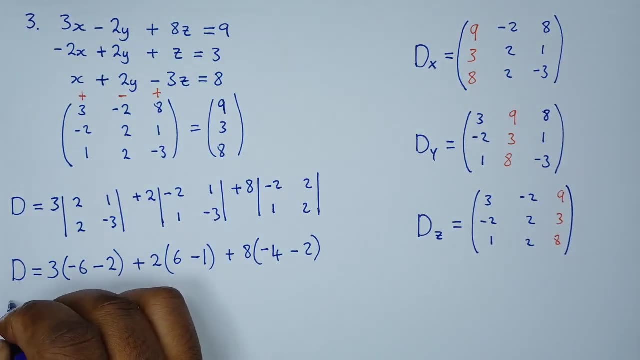 1 times 2,, of course, is simply 2.. So let's simplify. Simplifying this, what we're going to get will be: d is equal to 3, negative 8, plus 2, times 5, plus 8, times negative 6.. 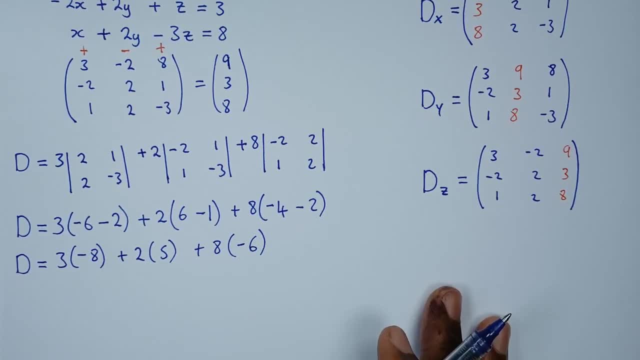 Like that, Let's proceed and find the value of d, So d will be equal to negative 24, plus 10, minus 48.. Like that, So it's very easy, and you'll avoid mistakes, if you, of course, do it step by step. 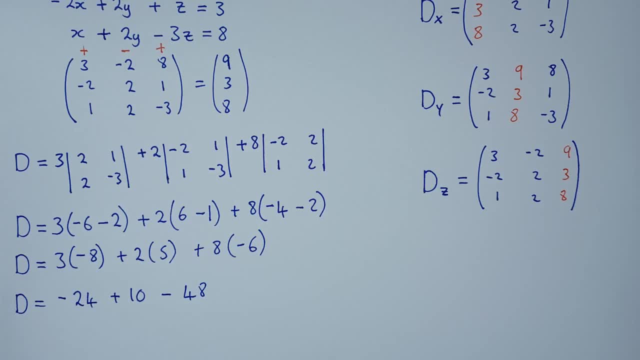 So negative 24, plus 10, minus 48. What we get is simply: the value of d is equal to negative 62.. Okay, So we have the value of d. So the next thing that we need to find is the value of dx. 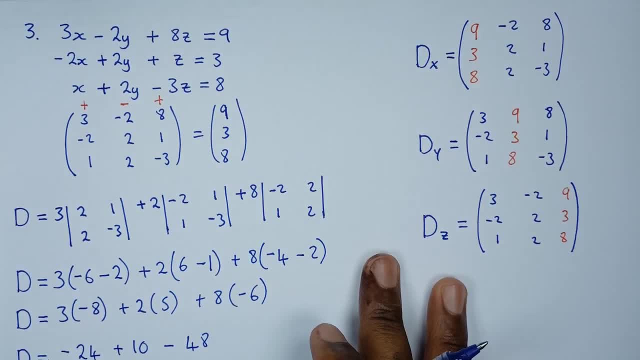 the value of dy as well as the value of dx, as well as the value of dx as well as the value of dz. So what we're going to do is I'll finish up this question, but for the next question, 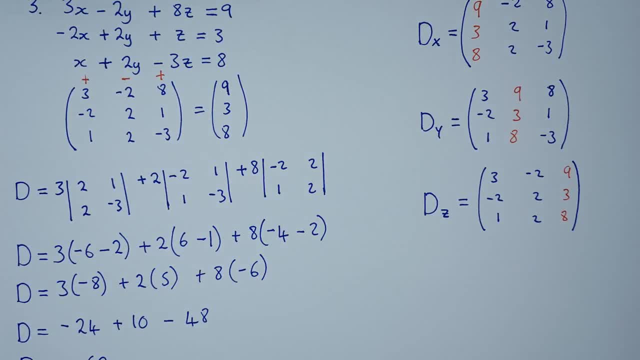 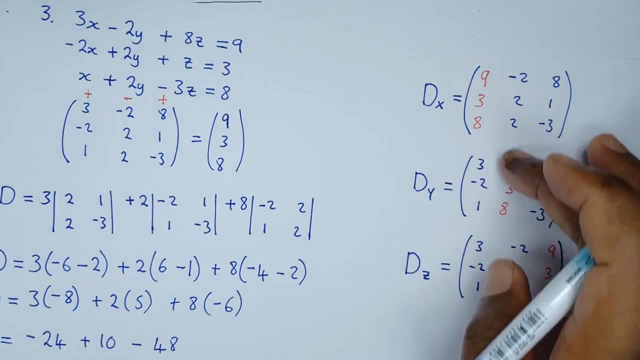 I'll just give you the values of the determinants and I'll request you to at least go through so that you find exactly what I'll find as well. So let's go ahead and find the three other determinants. So let's start with dx. 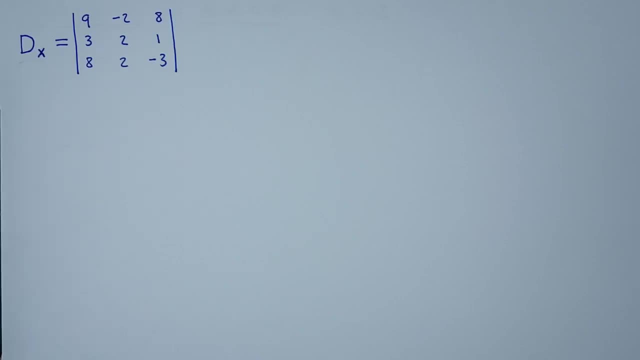 So we're going to do exactly what we did in the previous determinants. So this is a plus, This is a minus, This is a plus. Then the next step will be to list down everything that we have. So we have 9.. 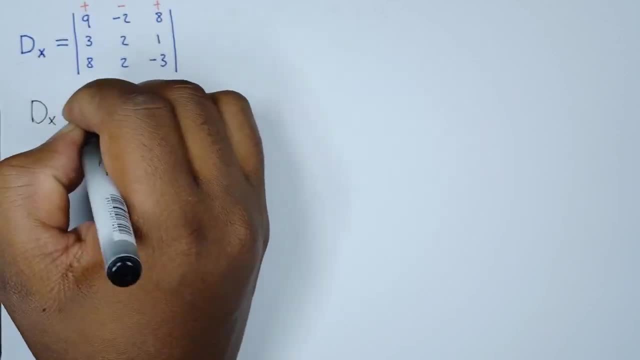 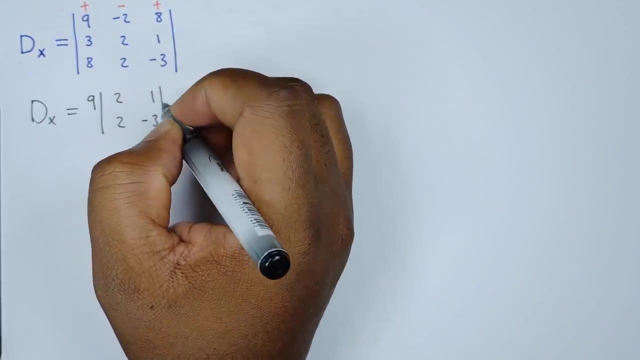 This is dx. We have 9.. The 2 by 2 formed will be 2, 1, 2, negative 3.. Then minus. So again there's a negative negative there. hence it will become a positive. 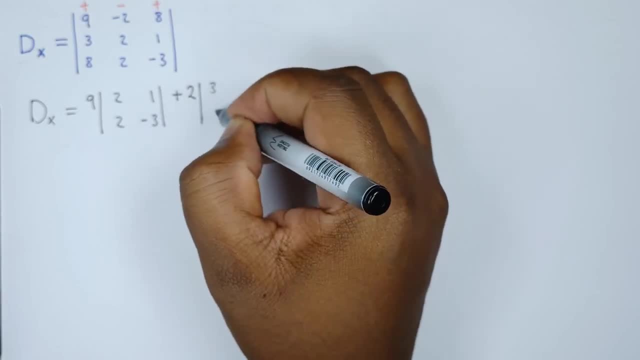 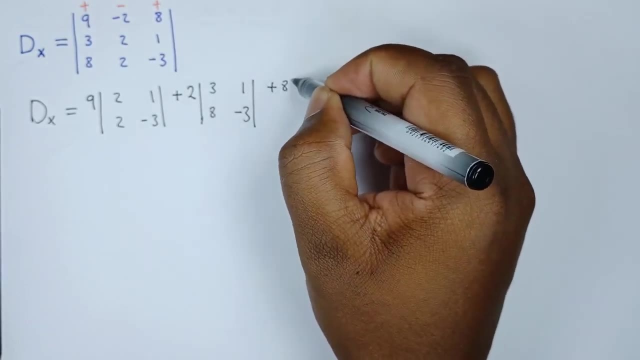 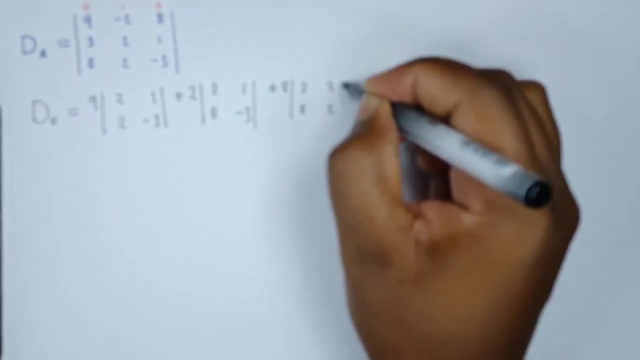 The 2 by 2 formed this time around will be 3,, 8,, 1,, 2, negative 3. Like that. And lastly, we have 8.. So 8,. the 2 by 2 formed will be 3,, 8,, 2, and 2.. 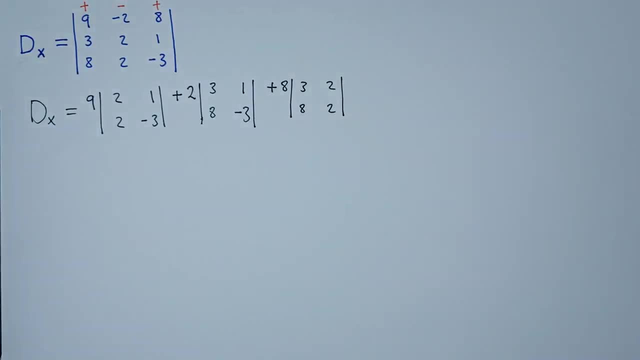 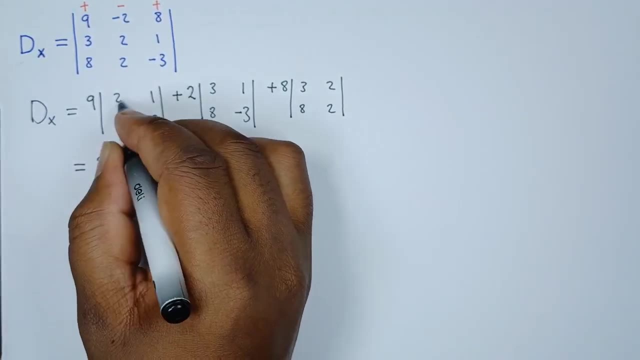 Okay, So now it's just a matter of finding the determinants of the 2 by 2s. So this should give us: we still have a 9 there. So that times that is negative 6 minus 2.. Then plus 2.. 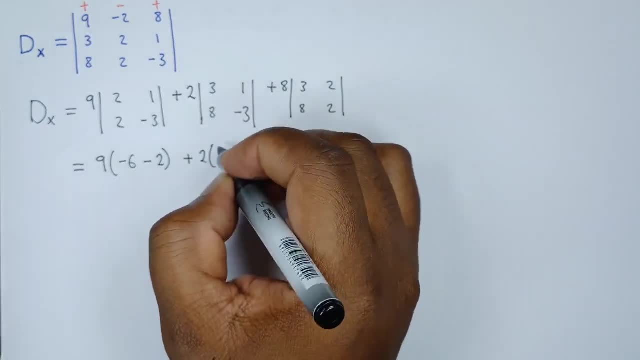 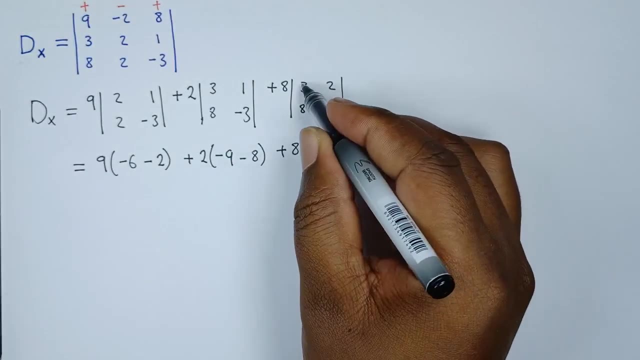 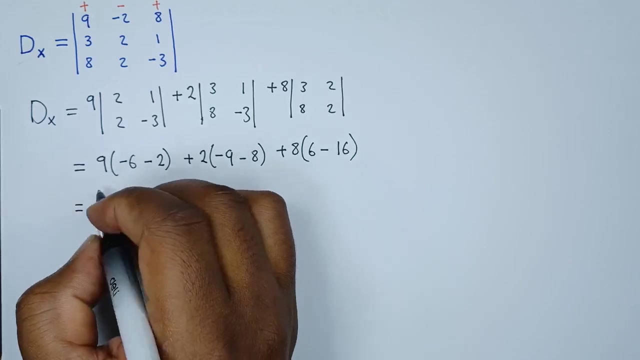 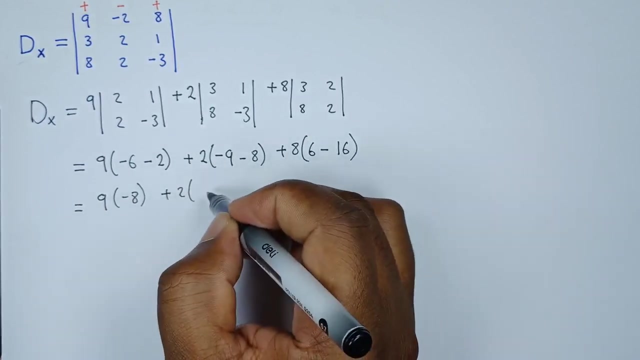 2 by 2 will be negative 9 minus 8.. And lastly, we have 8.. This will give us 6 minus 16,, like that. So the next thing we'll have will be 9 multiplied by negative 8 plus a 2, then here we'll have. 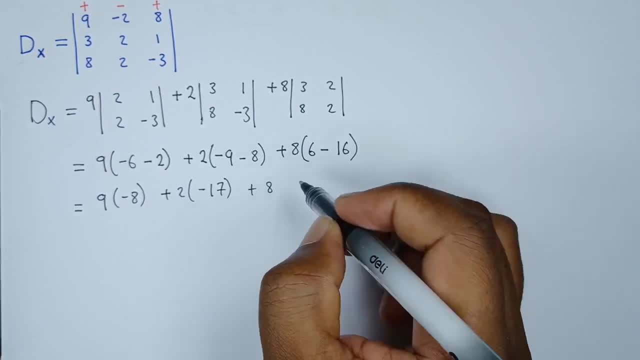 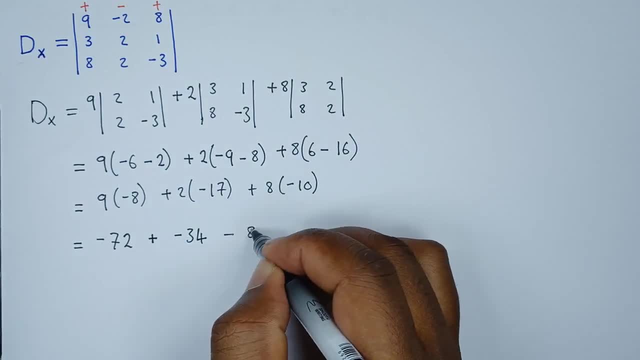 So if we put this equal to the negative 1, 2,, we'll get minus 1, 2, 3, 4.. Plus, So this and this will give us negative 84.. Like that, Then, lastly, that should give us negative 80.. 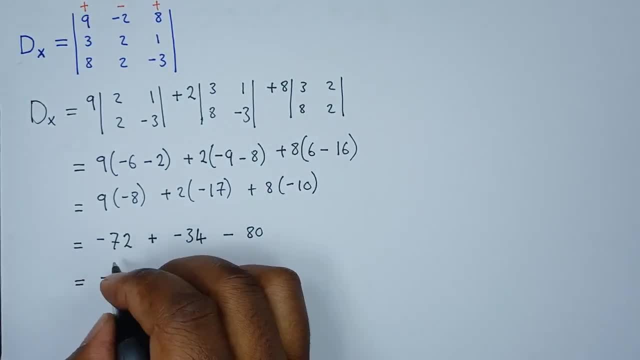 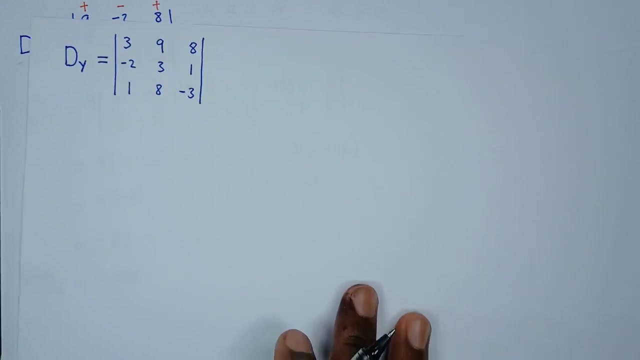 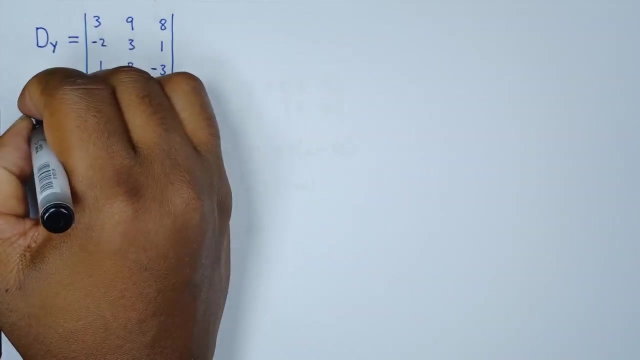 So adding everything together should give us negative 186.. So this is the value of dx. So we'll come and review everything. let's go ahead and find the value of dy. so the matrix for dy is this one that we have here. so let's find the determinant as well. so dy. 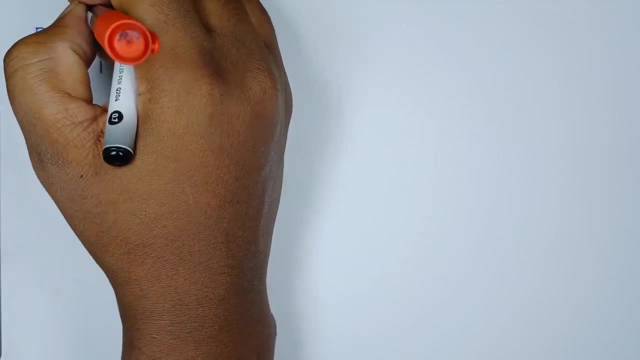 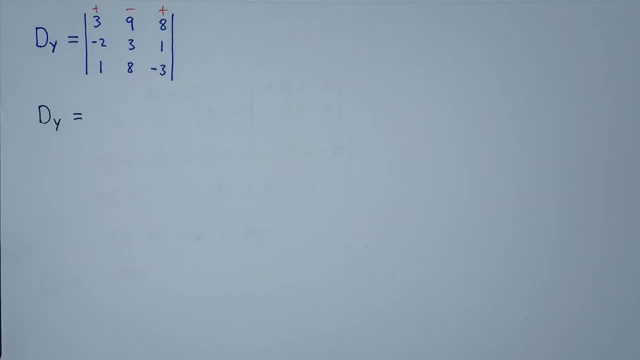 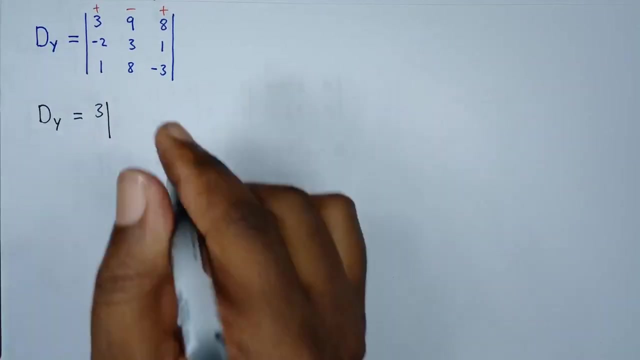 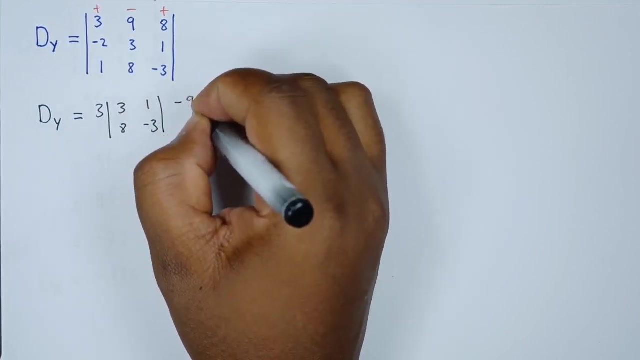 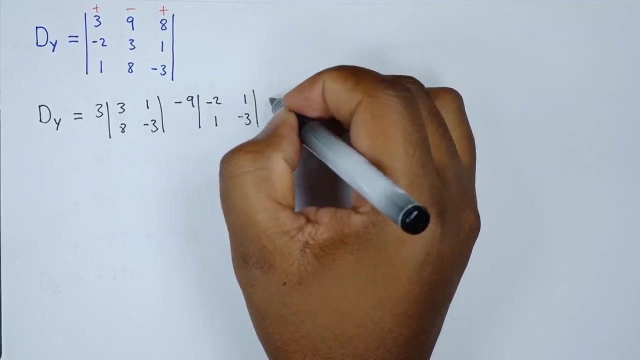 will be equals to. so applying the same concept where we say plus, minus, plus, so dy is equals to three. the two by two formed will be three, eight, one negative, three minus nine. the two by two formed will be negative two, one, one negative three. lastly, we have eight and the two by two forms. 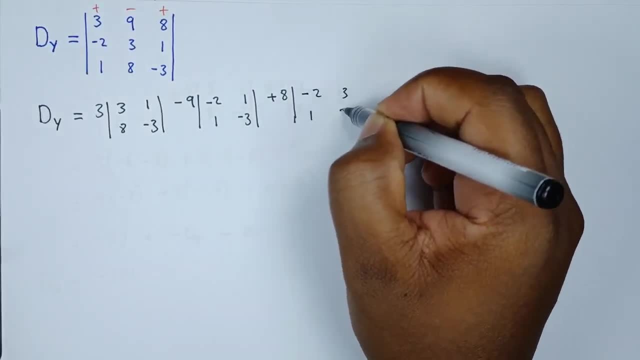 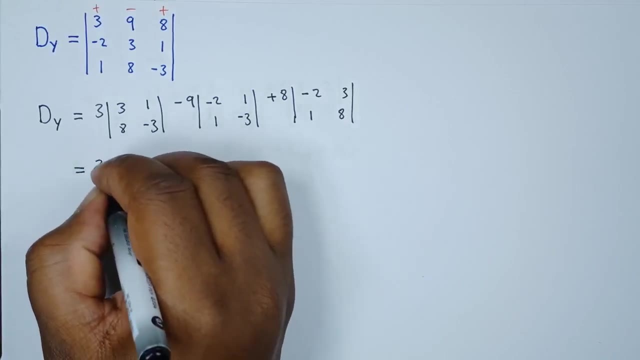 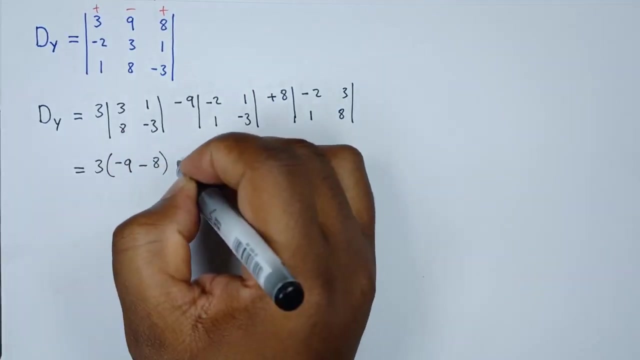 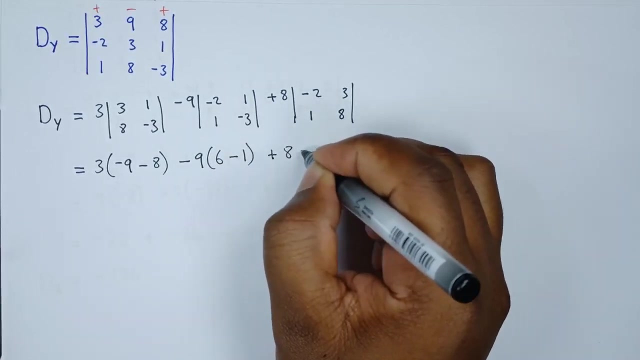 will be negative two, three, one and eight. so that's what we have. okay, so the next thing will be three. the determinant there will give us negative nine minus eight. minus nine. this will give us positive six minus one, then plus eight, this will give us negative sixteen. 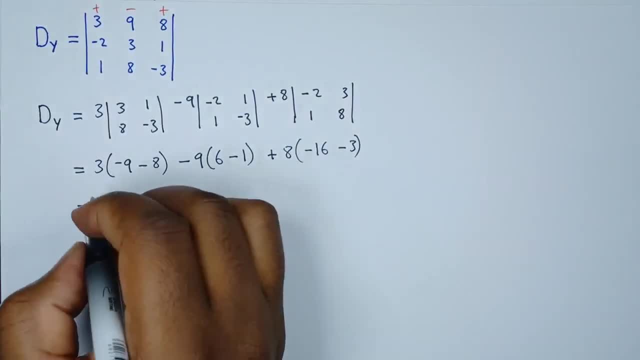 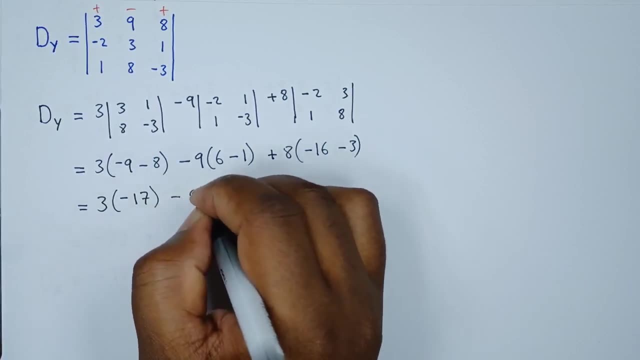 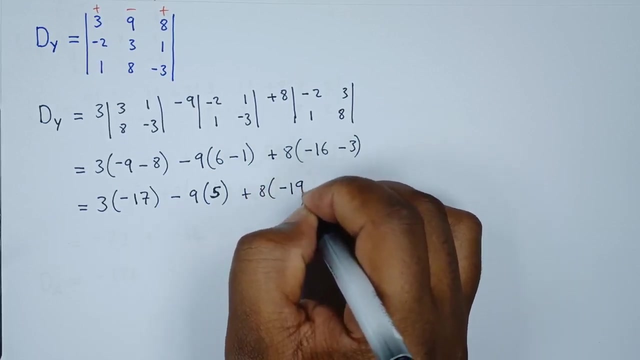 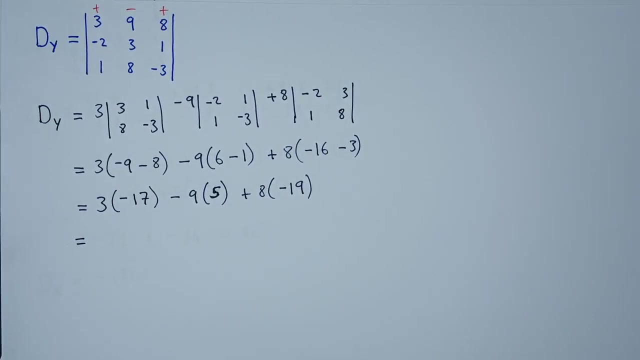 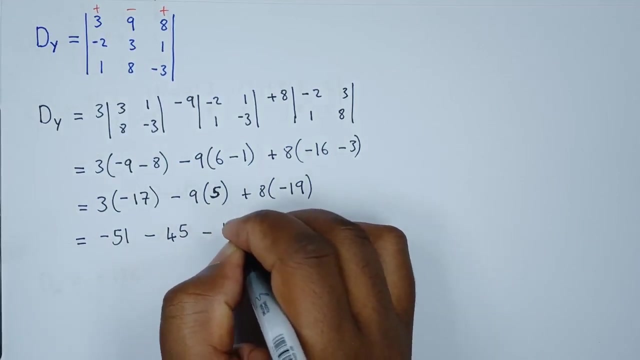 minus three, like that. so this will reduce to three. this is negative. seventeen minus nine, five by five. so five plus eight multiplied by nineteen- okay, so seventeen multiplied by three should give us 51 negative minus 45. then 19 by eight should give us a negative 152. so if we put everything together, 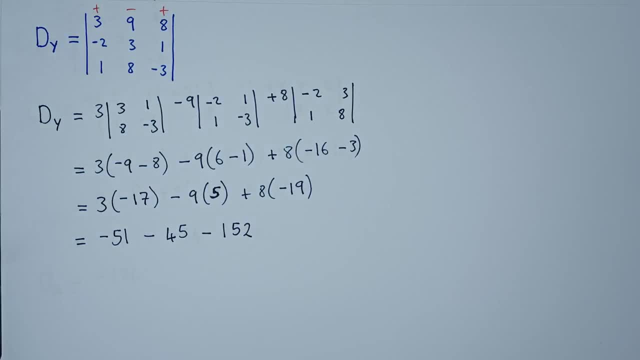 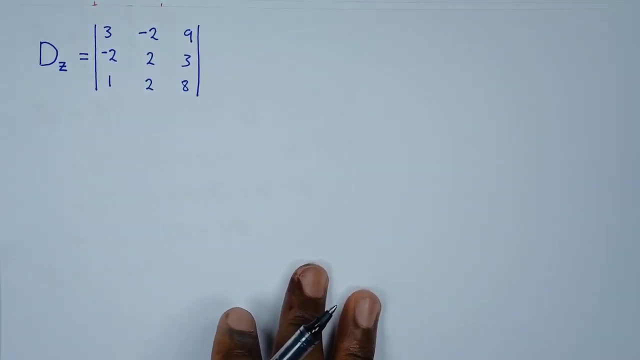 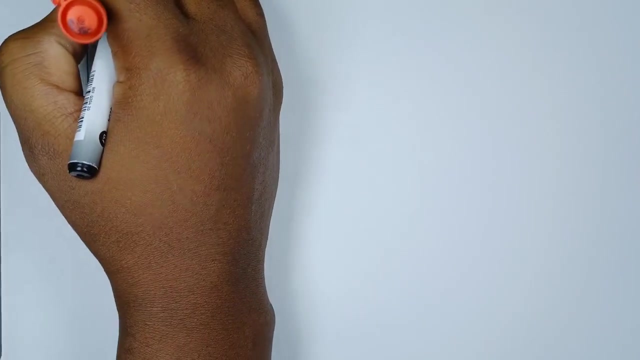 so 152 plus 45 plus 51, we are finding a negative 248. so this is the value of dy. so let's do the last part now, which is finding the value of dx. so this is the matrix that was formed by dz. sorry, not dx- same concept, this would be plus. 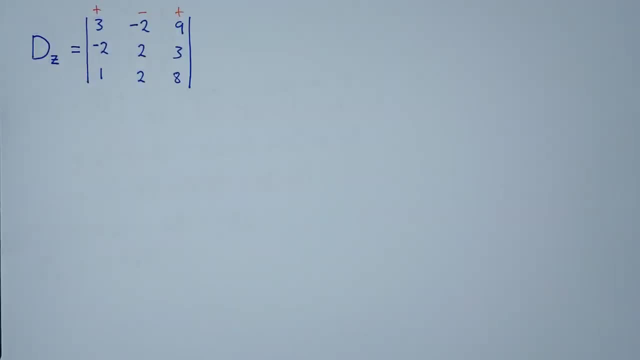 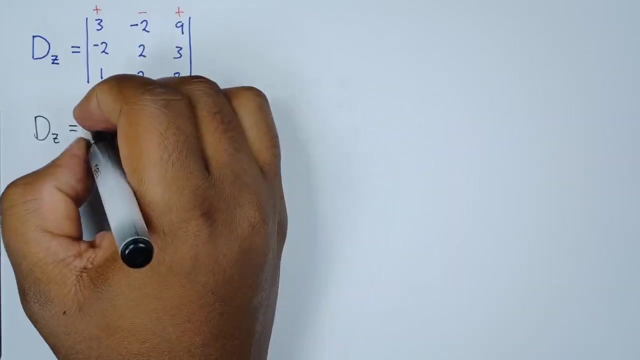 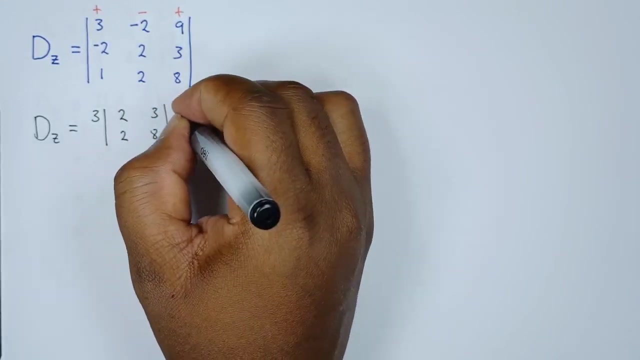 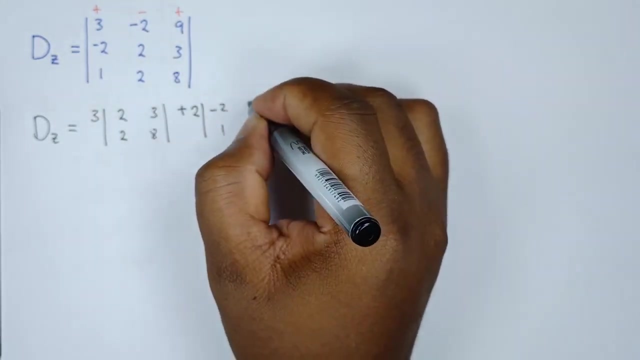 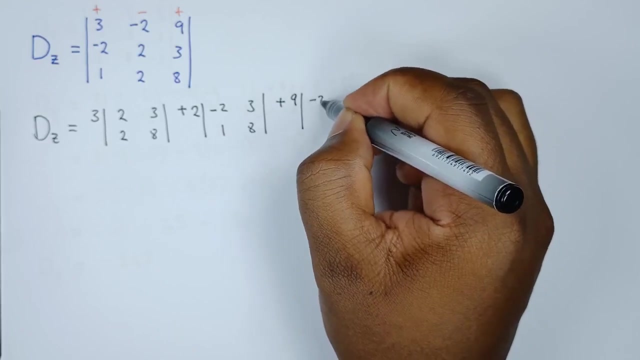 minus, plus. then from there, the next thing we're going to do is i'm going to say: dz is equals to three. two by two formed is two, two, three, eight like that, plus negative, negative two like that. so this is negative. two, one there, three there, eight there. the next part will be plus nine. the two by two form is negative two. 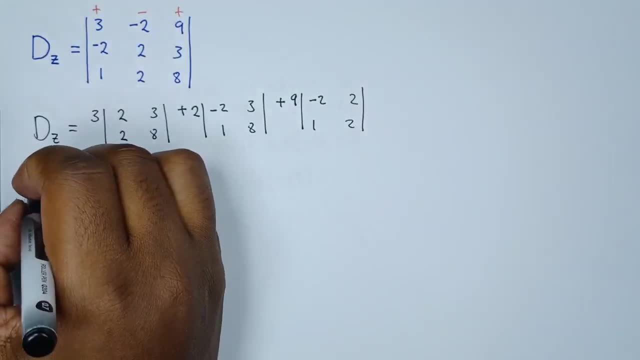 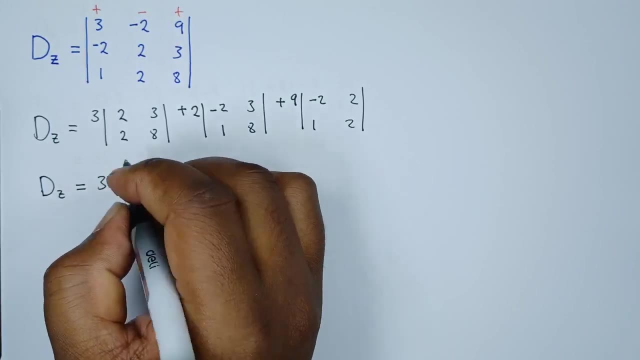 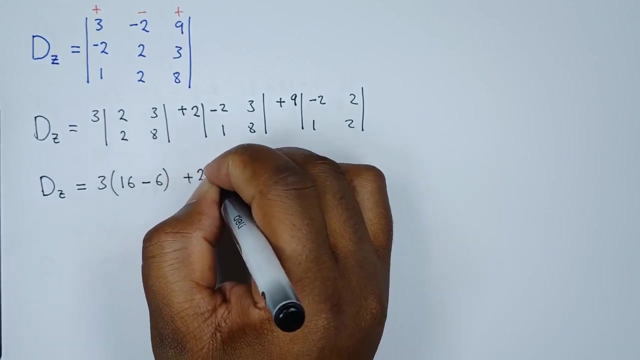 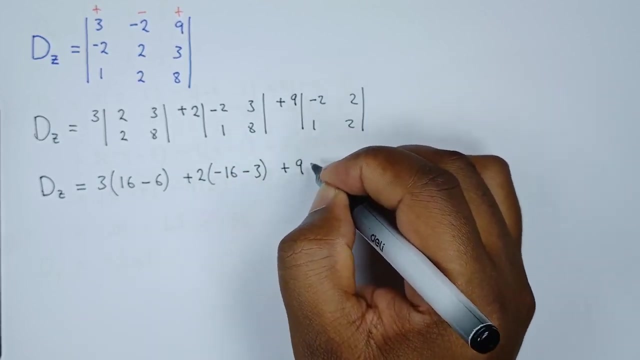 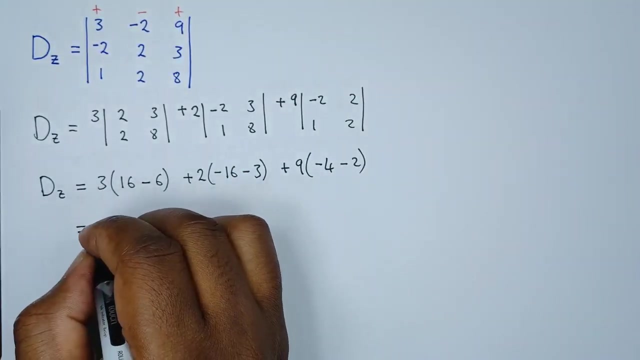 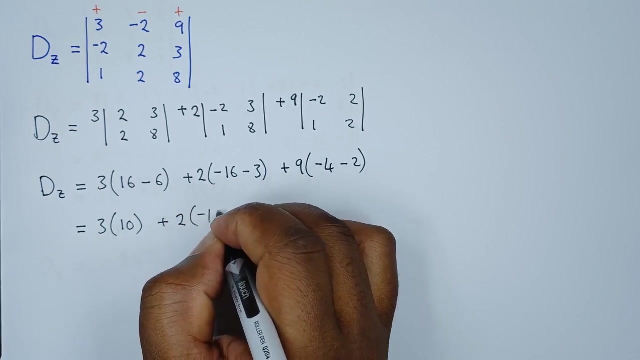 two, one and two. so dz will be equals to three. three. this will give us 16 minus six plus two. this will give us negative 16 minus three plus nine, and this will give us negative four minus two. so our dz will become three multiplied by ten plus two, multiplied by negative 19.. 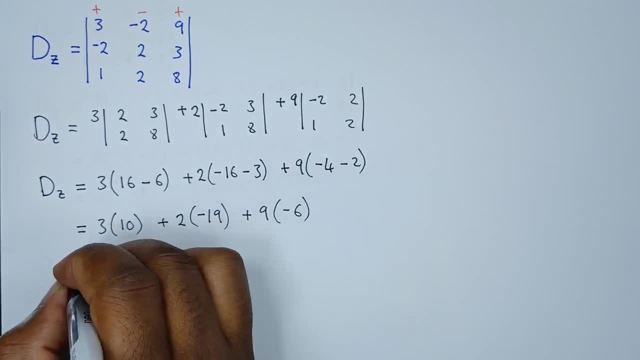 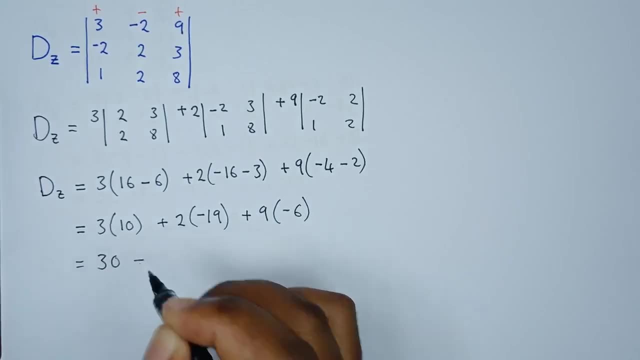 plus nine, multiplied by negative six. okay, so this, of course, will give us 30 minus, so 19, and two is 38, and then, uh, minus again. so we know that nine times six is a negative 54 in this case. so, putting everything together, which is 30 minus 38. 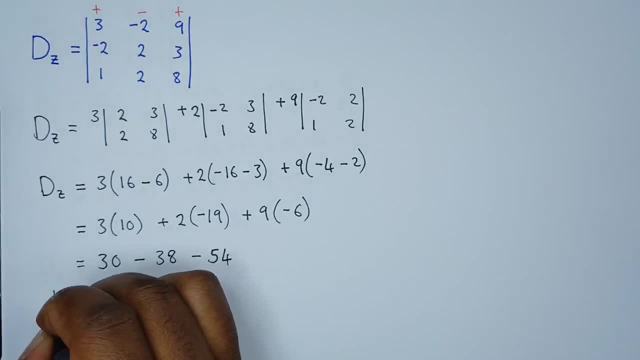 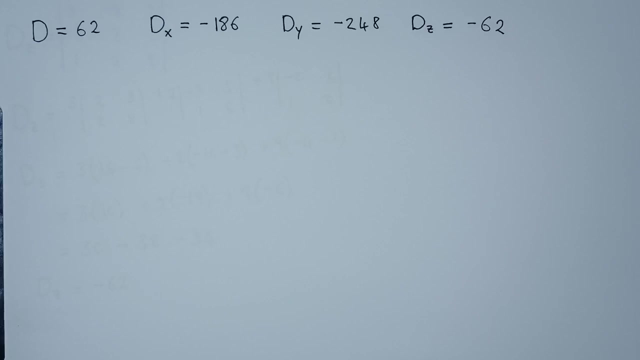 minus 54. what we get is simply: dz is equals to negative 62.. okay, so what we're going to do is we're going to review everything that we've found. so we find the values of x, y and z. so these are all the determinants that we've accumulated, so to find the value of x, x will be. 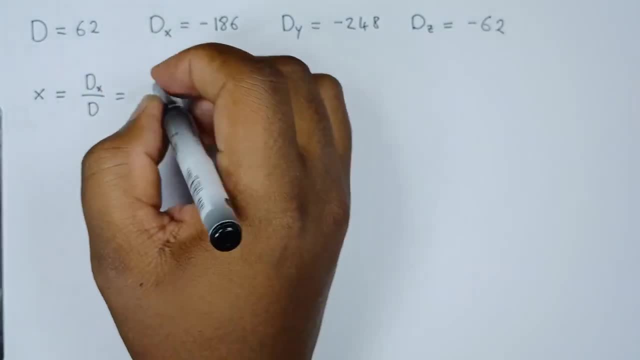 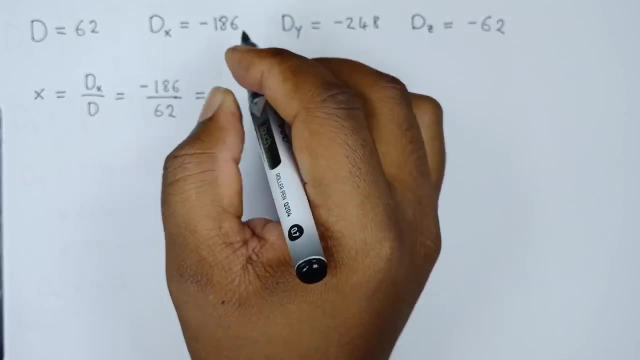 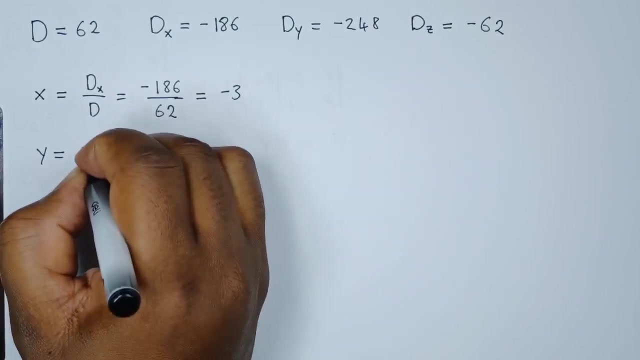 given by dx over d, our dx is negative 1, 86 or d is 62, so the value of x is simply negative. 3.. y is equals to. dys is negative two. sorry, let's write the formula dy over d, so our dy is two.